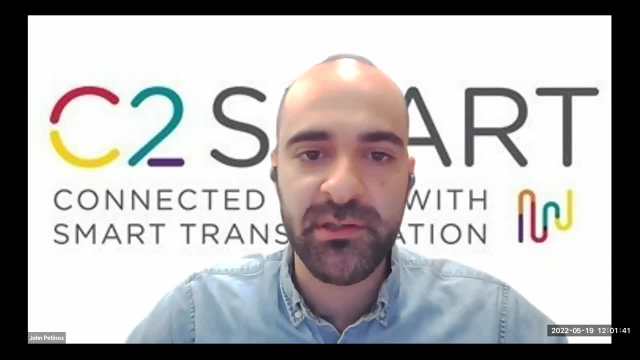 pressing urban mobility challenges. Just a few notes to start. We'll be recording this session, as you might have seen, and uploading it to the C2Smart Center YouTube channel. Questions make the webinar more exciting for me, you and the presenter, so I want to encourage. 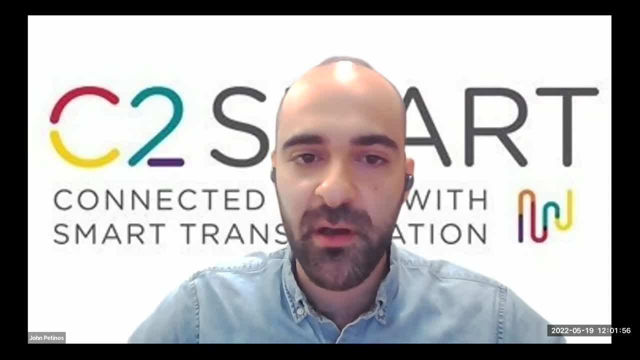 you to participate through posing questions, one of two ways. Either you can use the Q&A button at the bottom of the Zoom window or you can raise your hand. I'll unmute you and I'll allow you to ask your question directly to our presenter. Today I'm with Yiming Li. Yiming's a doctoral. 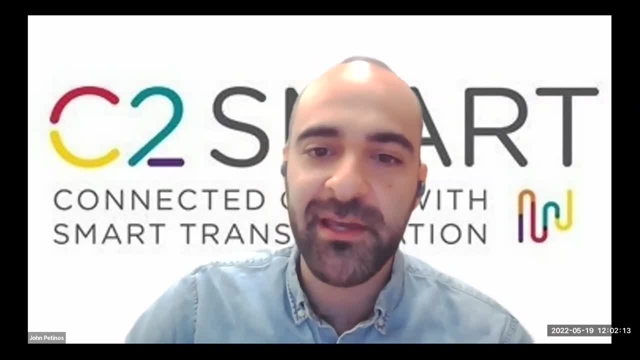 candidate in the AI Force Lab. It's AI Force CE at NYU's Tandon School of Engineering. His research interest is in the AI force lab and he's a professor at the C2Smart Center. He's a professor at the C2Smart Center. His research interests are in robot vision and learning with applications. 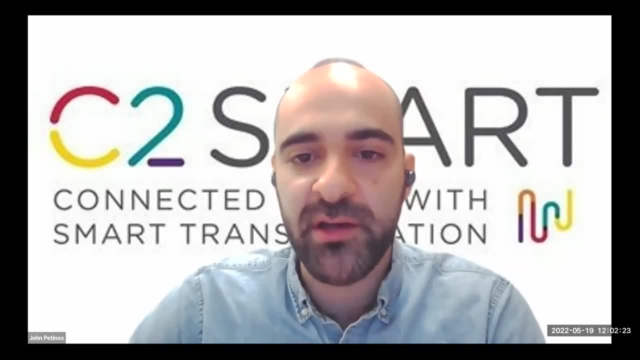 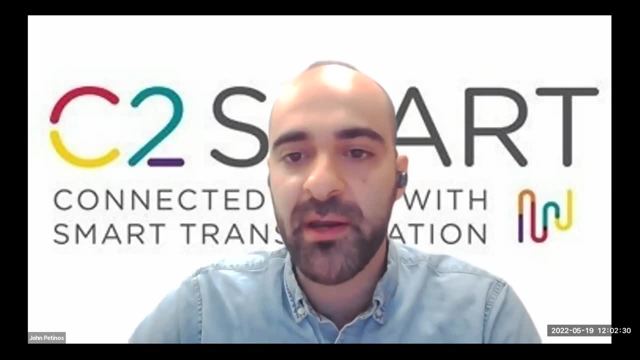 in cyber-physical systems, autonomous driving and human-robot interaction. Most specifically, he's interested in collaborative and adversarial perception, egocentric vision, multimodal perception and embodied AI. His works have been published in a number of top-tier conferences. 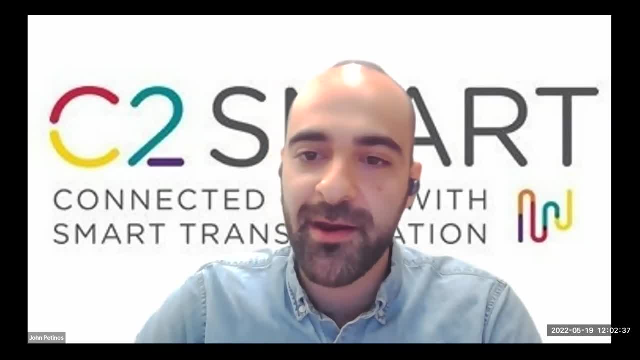 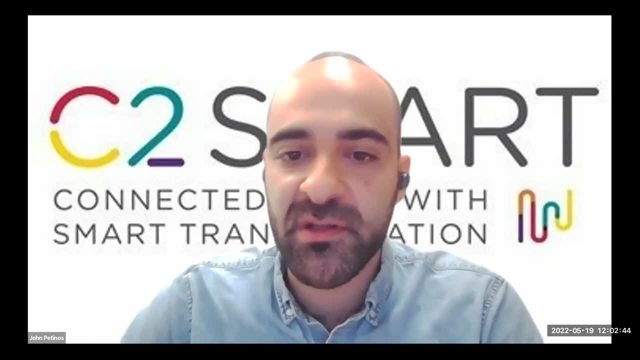 including NeurIPS, CVPR, ICCV, ICRA and IROS- a lot of acronyms. During his experience in his doctoral program, he's been able to visit the Mars Lab in the Institute for Interdisciplinary Information Sciences at Tsinghua University, Media Brain Group in the School of Electronic 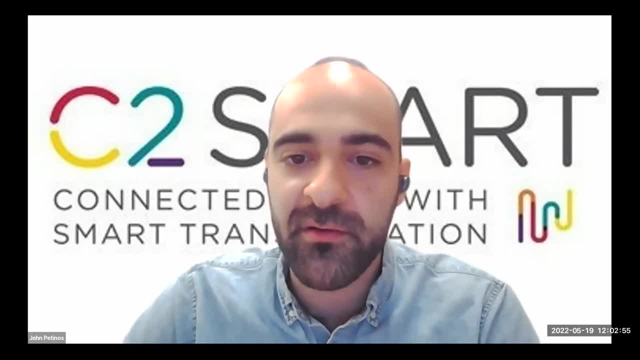 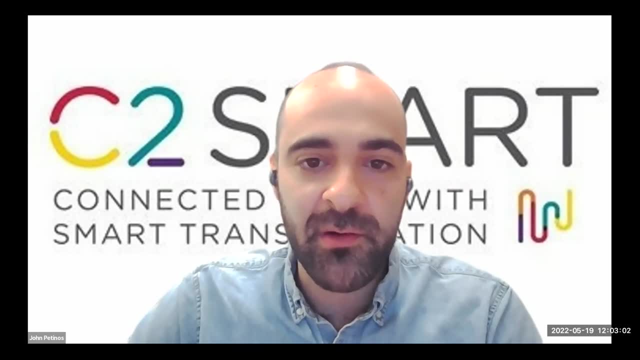 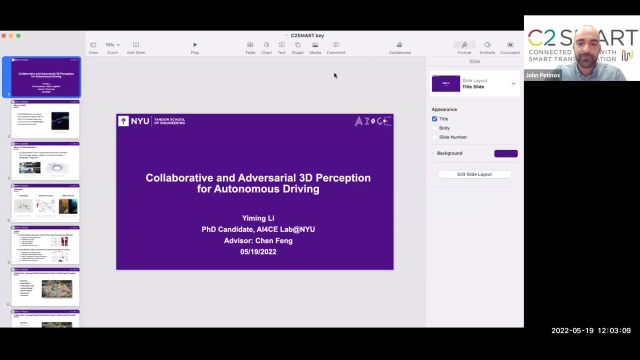 Information and Electrical Engineering at Shanghai Xiaotong University and the Institute for AI Industry Research at Tsinghua University. I guess, without further ado, Yiming, why don't you take it away? Hey, thank you, Let me share my screen. Can you see my screen now? Yep, yep, perfect Okay. 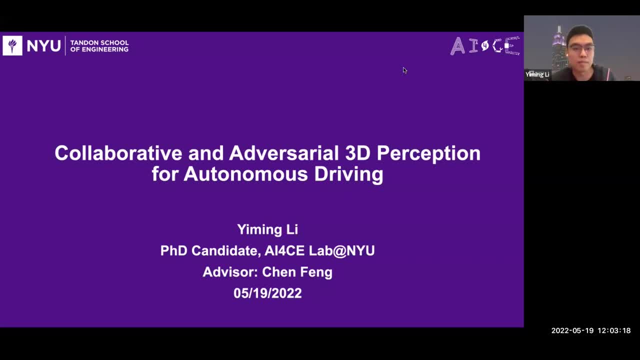 so let's start. Hi everyone, Thanks for coming to today's webinar, And I'm Yiming, a PhD candidate at the Air Force Lab at NYU, And today we are going to discuss the collaborative and adversarial 3D. 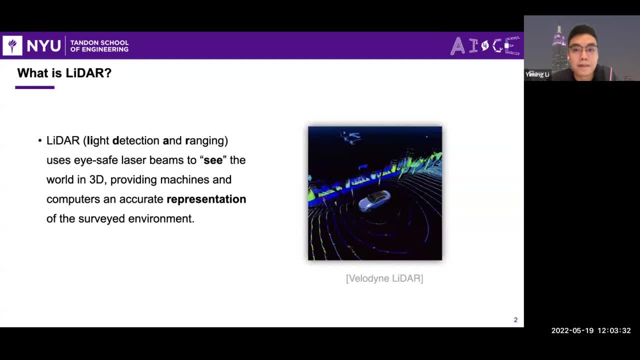 perception for autonomous driving And autonomous vehicles usually rely on 3D sensors to capture the 3D environments of the surrounding environment in order to achieve a comprehensive understanding of the environment, And we're going to talk about the 3D environment of the surrounding environment. 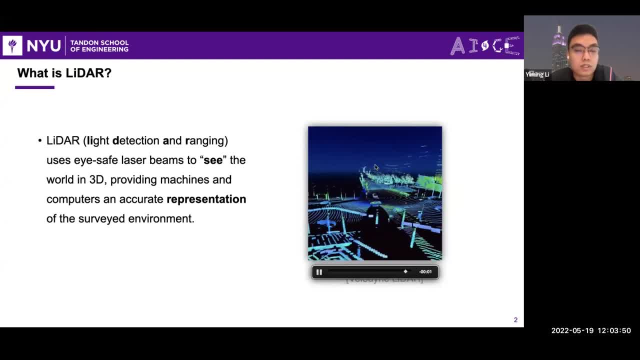 and why most key, why most important 3D sensors is LiDAR. And LiDAR shot is for light detection and ranging. It uses eye-safe laser beams to see the world in 3D And this can provide autonomous vehicles and accurate representations of the surrounding environment. And basically, LiDAR just. 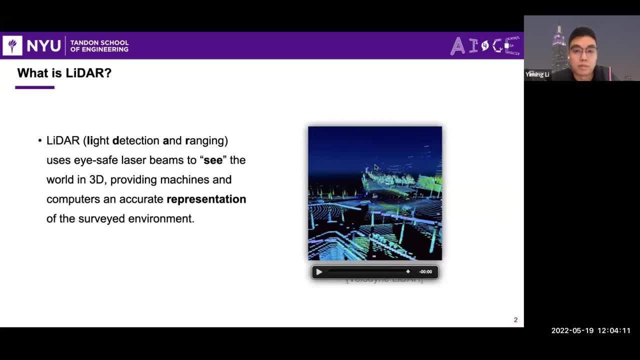 sends out some pulses of light which bounces off the object so that LiDAR can determine the distance between the object and the light. And so we're going to talk about the 3D environment of the surrounding environment, And after getting such kinds of 3D representation of the environment, 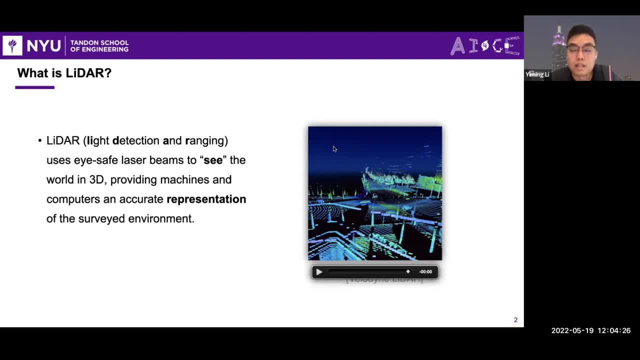 and the researchers usually use deep learning techniques to analyze the point cloud data and design some deep learning algorithms to capture, to process the captured point cloud data in order to achieve the comprehensive understanding of the environment. And today we are going to discuss one of the most important perceptions of the 3D environment, which is the 3D environment. 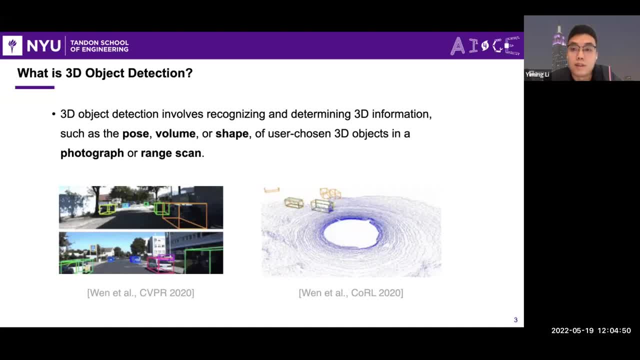 And we're going to talk about some of the most important perception tasks called 3D object detection. So what's the 3D object detection? And basically it just involves recognizing and determining the 3D information of some objects, some interested objects, for example, the vehicles, right And 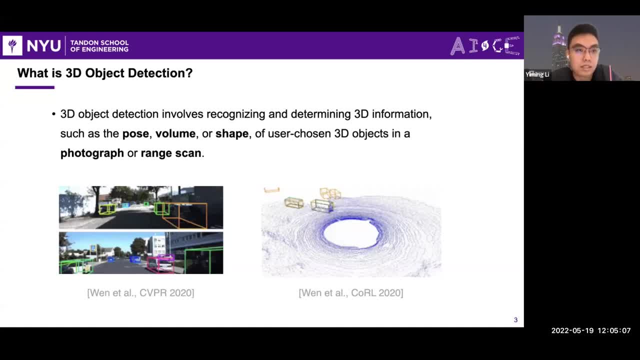 basically, you can understand the 3D object detection like we need to localize and draw some 3D bounding blocks, given some 3D objects, And so we're going to talk about some of the measurements. For example, the left figure shows that we need to localize the vehicles on a single. 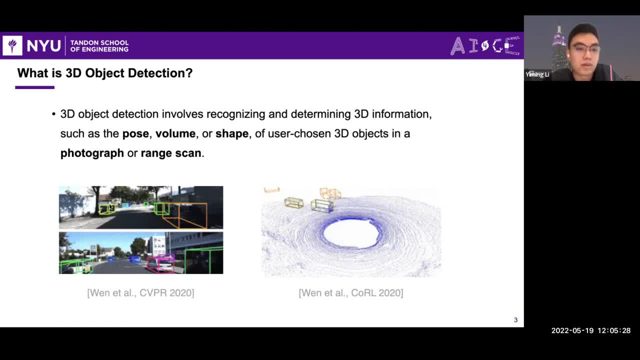 image You can see that we draw several bounding blocks, which is composed of the center's coordinate and the orientation of the bounding blocks and also the size of the bounding blocks, And also here the right figure denotes that we need to localize the 3D objects, given a single scan. 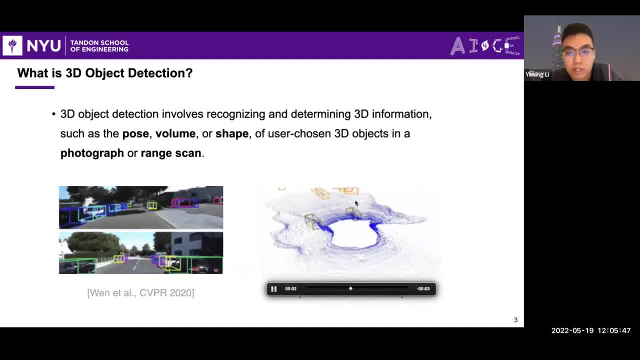 And you can see that we need to localize these objects. so we're only giving us 3D point cloud data And we need to localize these objects, And so today we are going to focus on the LIDAR-based 3D object. 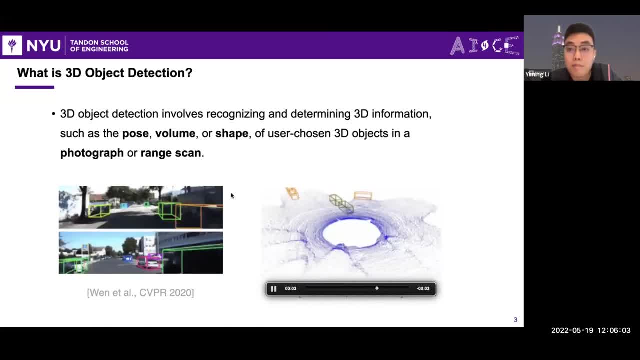 detection because for camera images, we will lose the depth information, And so for the LIDAR-based 3D detection, the performance is usually better than the camera-based object detection, And to process such a 3D object, we need to use the LIDAR based 3D detection to do these tasks. 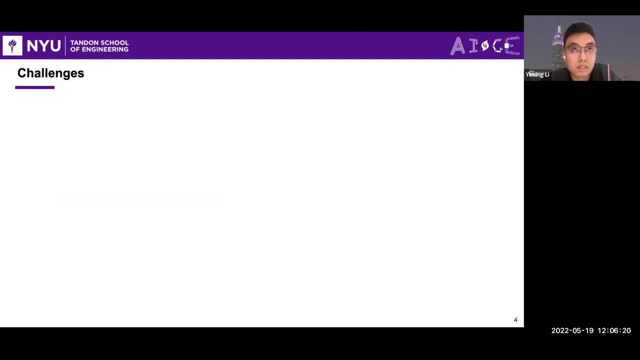 And to process such a 3D object. we need to use the LIDAR based 3D detection to do these tasks. kind of irregular data. and for point cloud, the basic understanding is that it is a set of points and, for example, given if one same level point cloud has n points and then it will be a 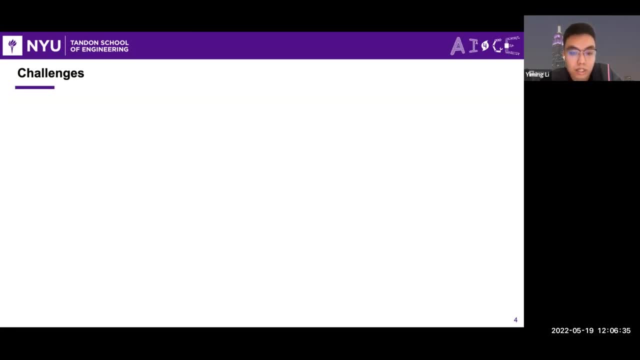 multiplied three matrix, and also the each row denotes the xyz position of each point, and we need to process such kind of irregular data. and there are several challenges in processing such kind of data with deep learning techniques. the first one is data sparsity and this is because of the limited sensing capability of the 3d lidar. so 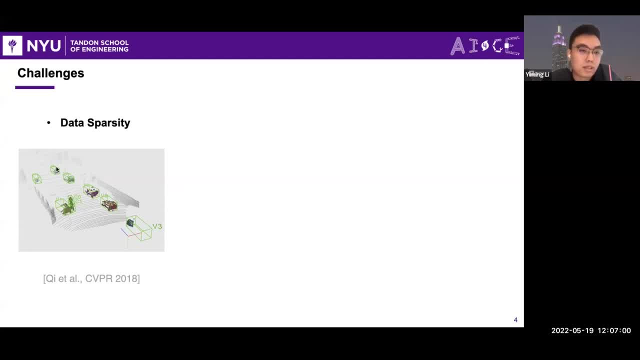 they are usually really sparse measurements when the object is far away from the lidar. you can see that here this point denotes the, denotes the ego vehicle, and you can see that this object is quite far, far away from the lidar. so there will be fewer measurements compared. 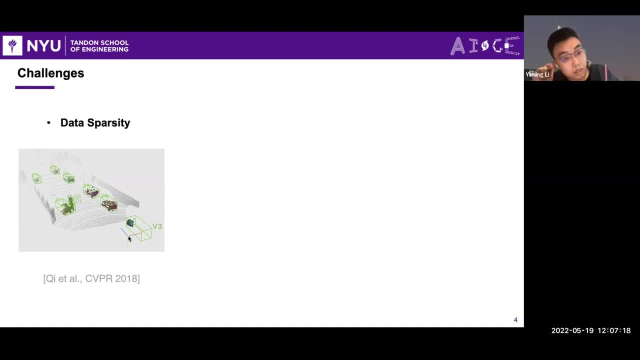 with objects which is closer to the lidar. so if we have very scarce, very sparse information on that object, so the algorithm will be. it is quite challenging for algorithms to localize such kind of object. and the second challenge is partial or full occlusion because of the this, this: 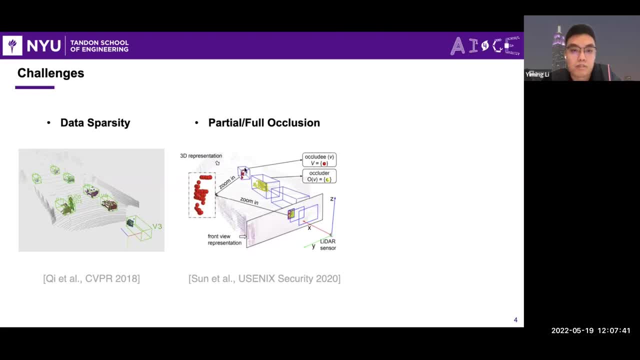 challenge is because of the dramatic relationship. for example, here the red the, the bunny box with the red dots, denotes, denotes an occludy, and this is: this object is occluded by this yellow object and so, due to the occlusion, there will be also sparse measurements, sparse or fewer measurements. 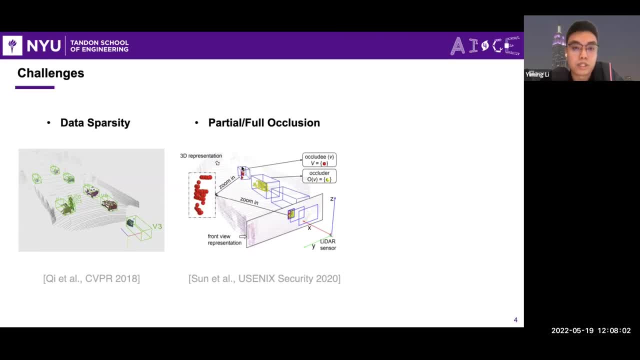 of that object and or even sometimes this object is fully occluded by by the other, by the other vehicles. and the third challenging is the motion distortion. this, this is because of the uh lidar's property, because uh lidar is rotating uh during the measurement, measurement capture and 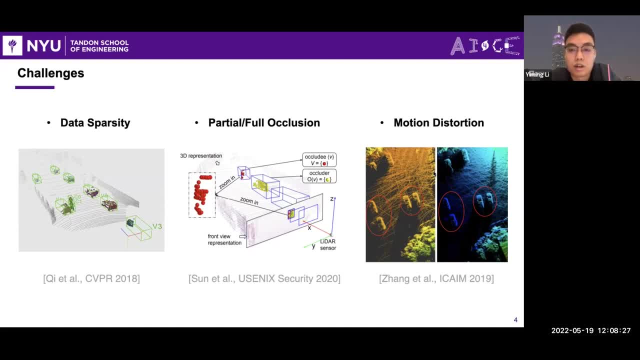 so, and the lidar which is attached to the autonomous vehicles, uh, is still, is still moving, when it when it rotates. so the different measurements will be captured at different time steps and also at different locations. so these measurements actually need to be synchronized. the unified coordinate, if, uh, if. 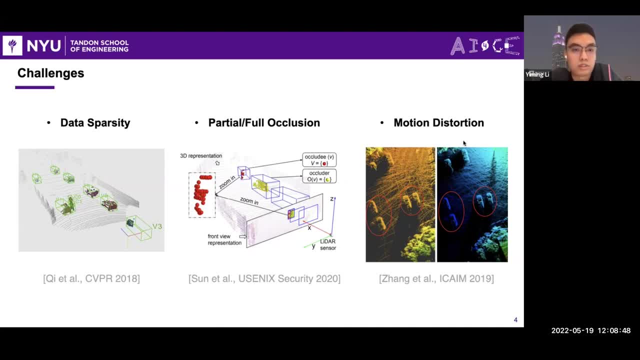 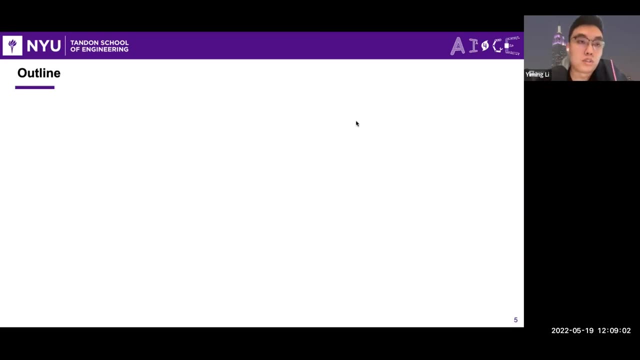 we do not have accurate pose, then this will introduce the motion distortion. so with this, uh, these challenges, then today i will, then i will show you how we design uh novel deep learning algorithms uh to process such kind of 3d point cloud data in order to 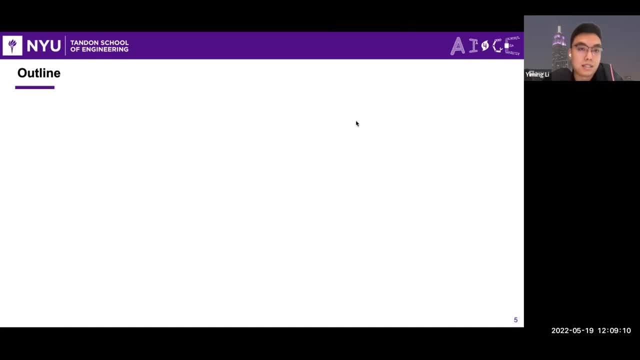 achieve uh robust 3d perception, and today i'm going to discuss from two aspects. the first one is collaborative And I were going to introduce our works published in Europe's 2021, which named us learning distilled collaboration graph for multiagent perception, And in this work, we our main contribution. 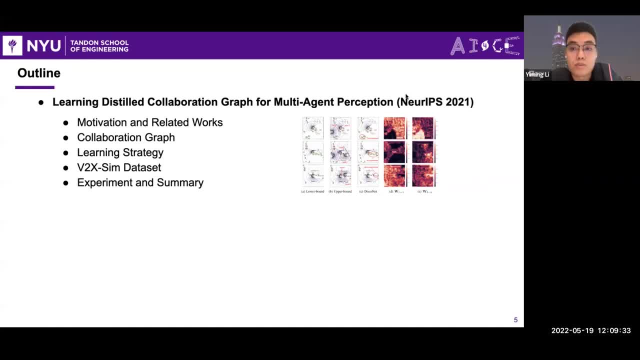 is. we propose a collaboration graph with matrix, validate weight, And we also propose a new learning strategy which is based on the knowledge distillation to learn such kind of graph. So with such kind of graph, the agent, the ego, vehicle could understand which part. 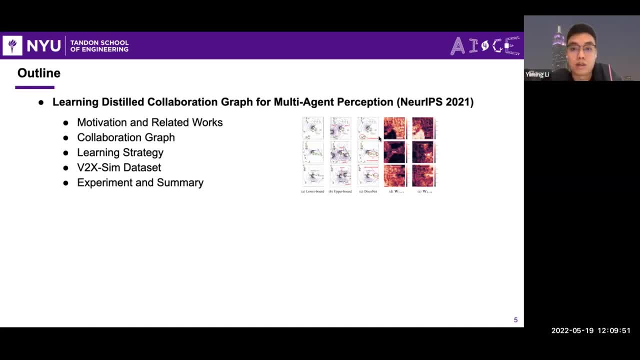 which spatial range need, need the information and which spatial range has no, with noisy information needs to be repressed. And our second, second work is from the advert, adversarial perspective And in this work, named as fully light up perception, the adverse trajectory, preservation, we 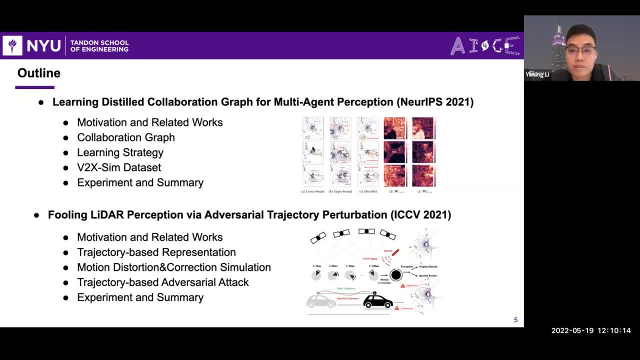 propose. we propose the trajectory based at a virtual attack framework against a lighter based perception And which which we revealed an overlooked vulnerability which lies in motion motion compensation process And we also show that and very perceptible motivation introductory will hurt the 3d detection performance. Okay now. 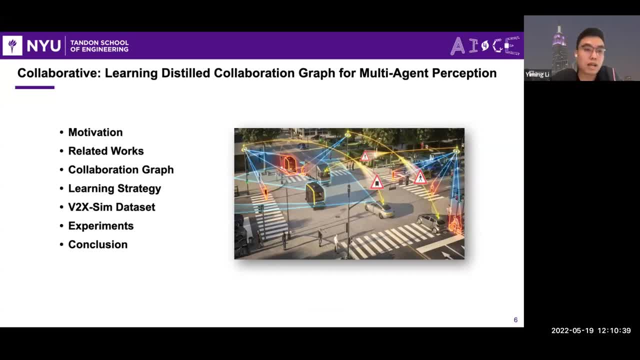 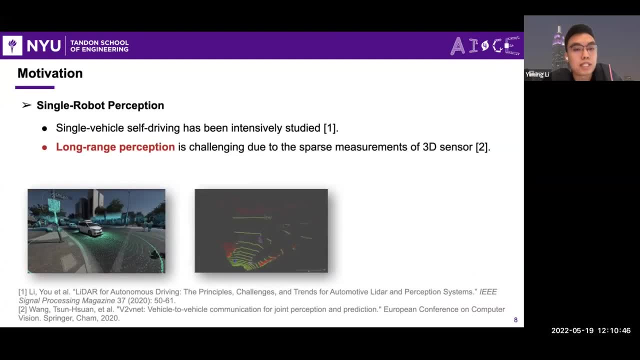 let's start with the first one: collaborative, collaborative, collaborative, collaborative part. As I mentioned before, the single robot perception, although it has been widely studied and various algorithms had been proposed to process that kind of kind of data. Then, however, the large issue is is very challenging due to sparse measurements at a long distance And also there is frequent occlusions due to the individual viewpoints here. you can see that in the right figure. 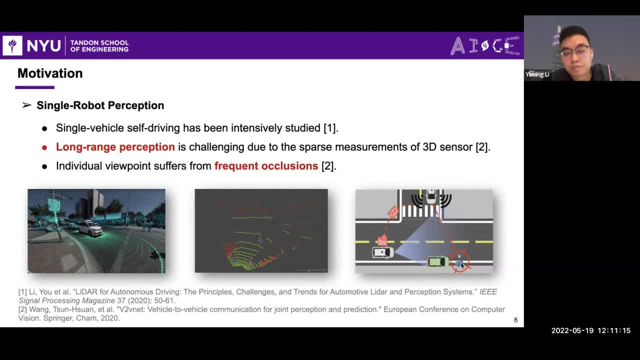 the ego vehicle tries to perceive the this person. however, due to the occlusion caused by this green vehicle, it is hardly to. it is very, very, very challenging for it to perceive this this person. However, with with such kind of vehicle to vehicle collaboration, you can see that the top part has a white vehicle and it can perceive the person better. And so that after such kind of message, message sharing, then the, the, the, the, 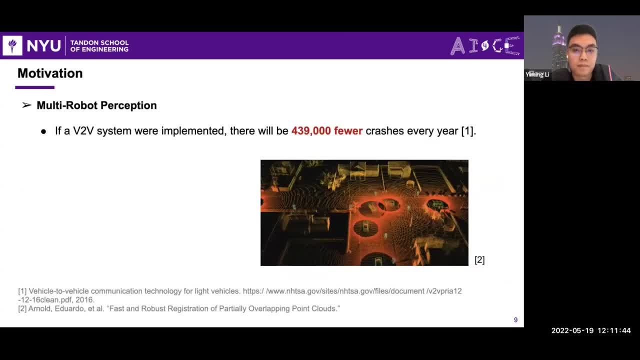 perception robustness could be improved. So, as I just said, the multi-robot perception has been proposed to solve the issues of long-range perception and frequent occlusions and, according to the estimation of the US Department of Transportation, if a vehicle-to-vehicle system were implemented, 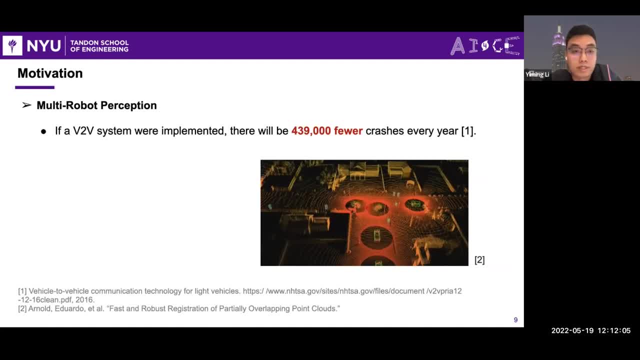 there will be around 440,000 fuel craters every year, And there are two main advantages for the vehicle-to-vehicle system, And the first one is there will be more viewpoints. So this is quite useful for the perception, because you will have more information right. 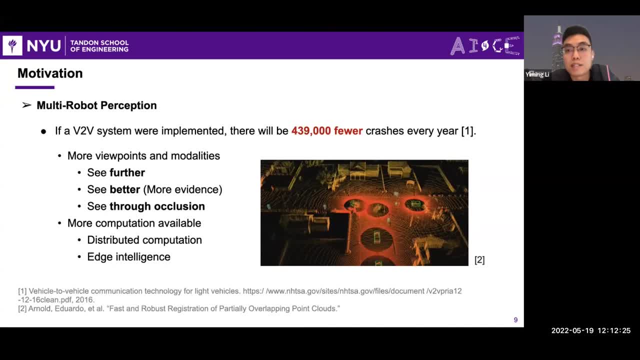 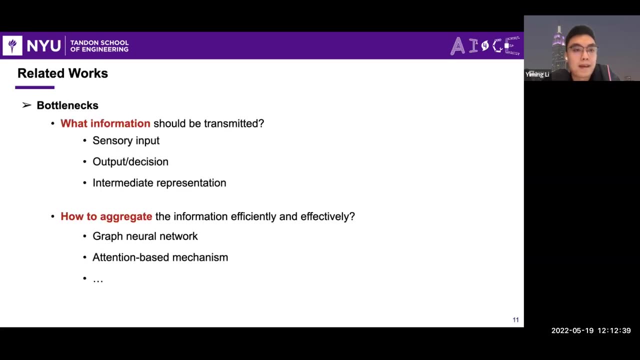 So the vehicle, so the vehicle could see further, see better and even see through occlusion. And also you have more computational resources in your whole perception system and this will also improve the efficiency of the whole perception system. And two: 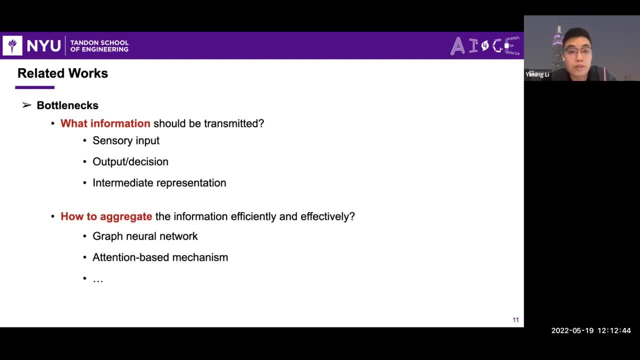 to design such kind of robust collaborative perception framework. there are several questions to be answered. The first one is what information should be transmitted right, And also the second one is how the vehicle aggregates the information from the other neighboring agents efficiently and effectively. 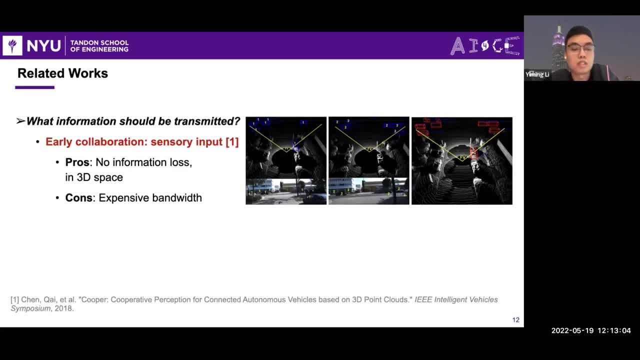 As for the first question, there are several solutions, For example, the first one is early collaboration. Some researchers just aggregate all the raw point cloud data in the Euclidean space and then start to process that kind of aggregated data And such kind of early collaboration. 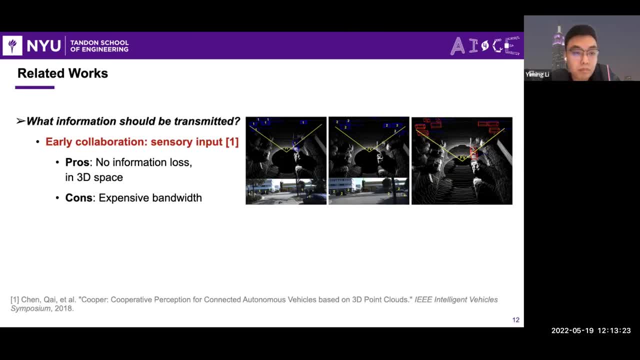 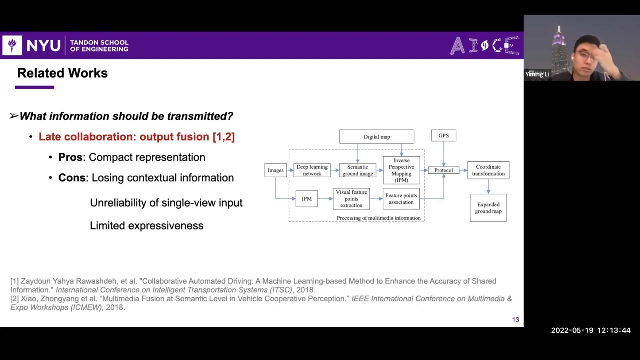 has no information loss, so the performance is very good. However, the communication bandwidth is quite expensive because generally for same level point cloud, it has a lot of points and this will lead to a very expensive communication bandwidth And also some researchers propose late collaboration. 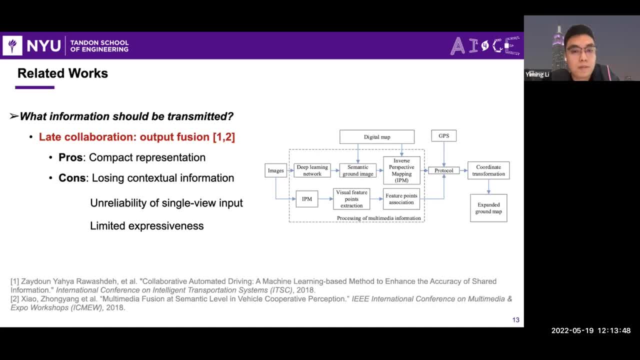 which is just fuse outputs of each vehicle. However, although this kind of method has a cheaper communication bandwidth, however, each vehicle with its own individual viewpoints cannot have a very good perception results. Also, this leads to the unreliable results because here we just fuse several outputs from different 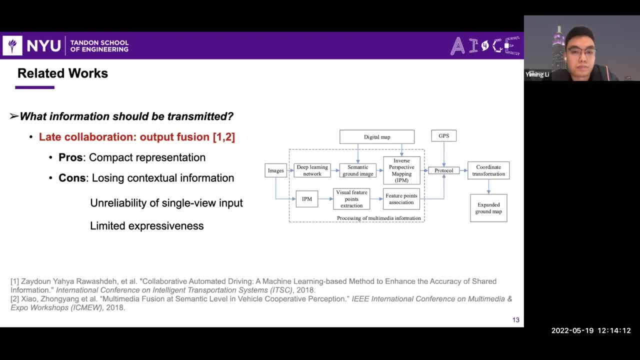 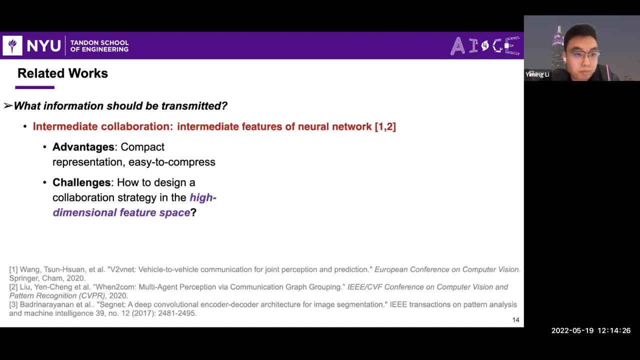 you know, different outputs And from different individual agents, And each individual agent has unreliable results. And the fusion of unreliable results cannot result in a robust perception performance. And recently deep learning has been widely applied in 3D computer vision, And so researchers in the collaborative perception direction. 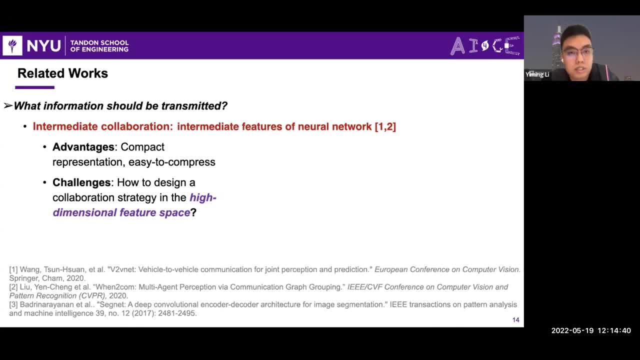 and they try to think about how to utilize the deep learning in this collaborative perception setting. And they propose, instead of fusing the early, the raw data, fusing the output. instead of fusing the input and fusing the output, they propose to fuse the intermediate representations. 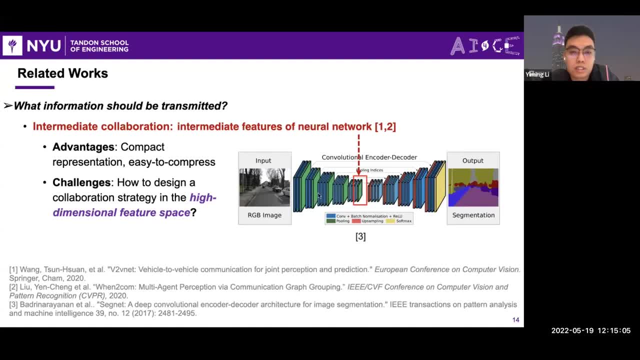 of your network, So that this results in two kind of advantages. The first one is this representation is compact and easy to compress, so that this can help us to reduce the communication bandwidth. The second performance, second advantage, is that here now we are still having some contextual information right. 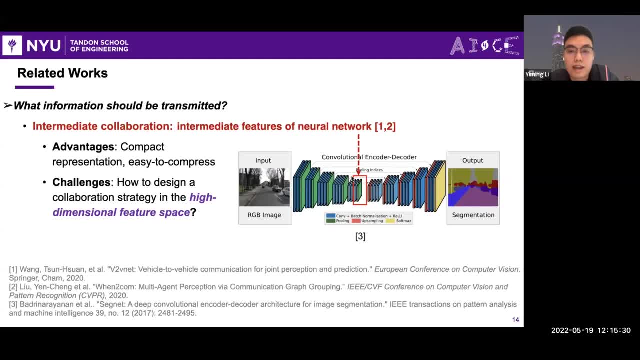 And this can also if we have a very, very well designed communication modules, then these representations can help us to achieve the comparable performance with the input-based fusion, but with very, very low communication bandwidth. So the challenge is now how to design a collaboration. 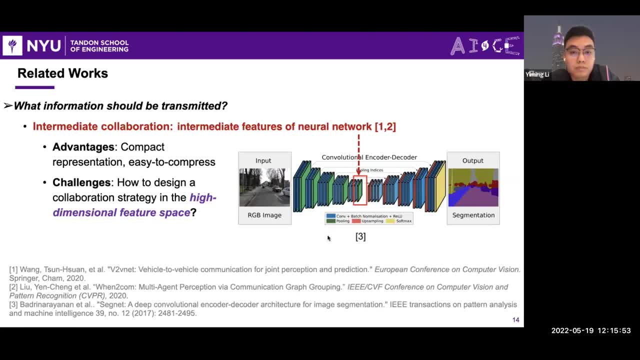 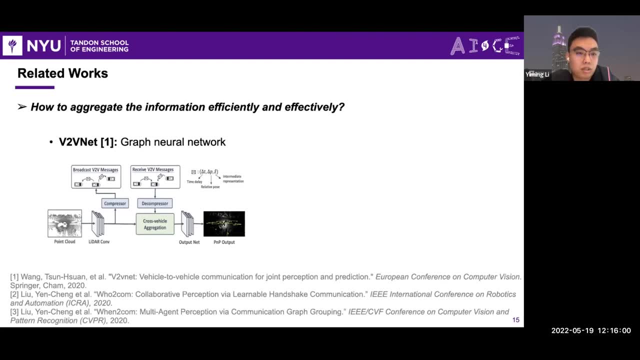 strategy in the high-dimensional feature space, And researchers had proposed several kinds of strategies. For example, the Uber Autonomous Driving Group had proposed to use a graph neural network to model the collaboration among different agents, And in this graph each node denotes a ego vehicle. 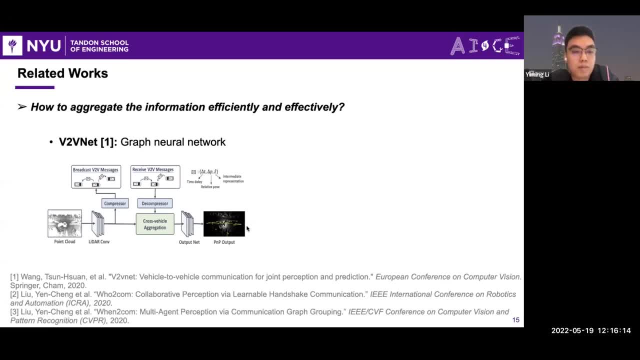 and they use graph neural message passing to propagate the information in this collaboration graph. And also several researchers proposed to use a tension-based mechanism to aggregate the information. For example, they use here who2come used a tension-based mechanism to select the collaboration partners. 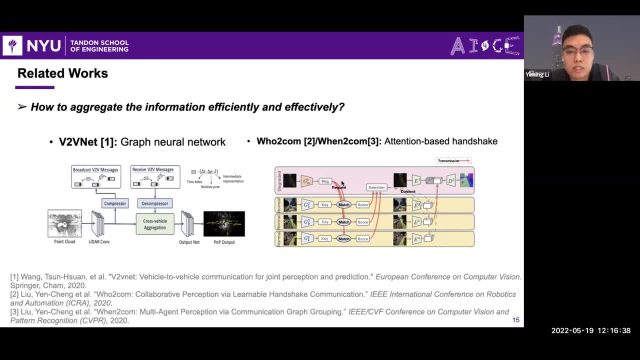 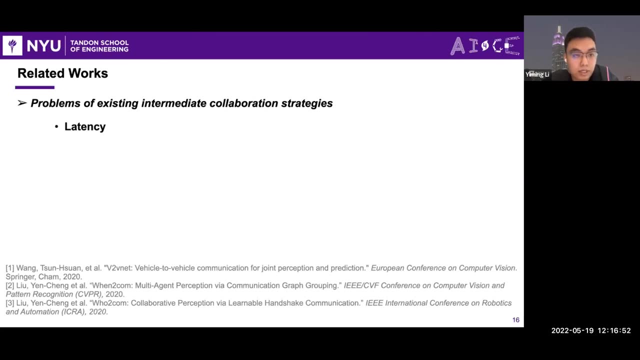 And basically the idea is that if one agent which has information, which has a higher correlation score with the ego agent, and then it will be selected as a collaboration partner. And, however, some problems still exist, For example the latency problem. 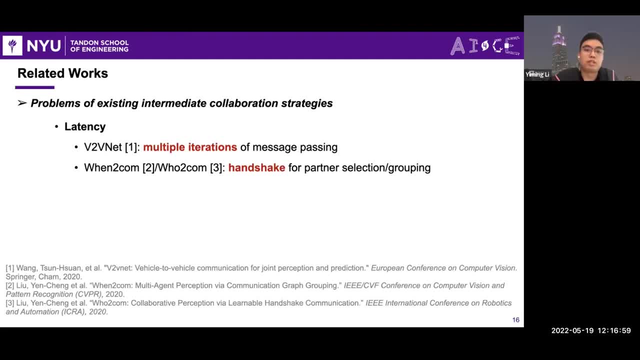 v2vnet and who2come both needs multiple iterations of master passing and this will introduce the latency problem. And the second problem is accuracy And also each ego vehicles. their message has a spatial resolution right, Because this message, it covers a certain area. 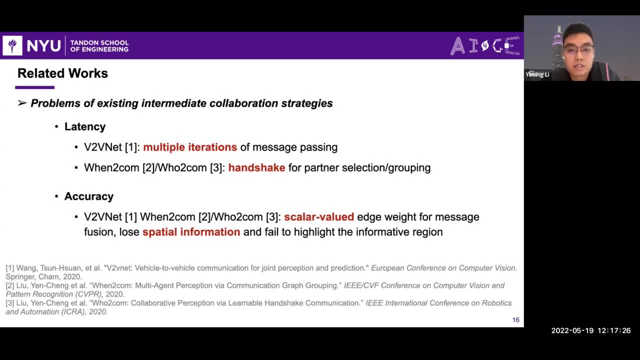 So it definitely has a spatial resolution. However, these methods consider a single-valued age weight for message fusion. It just uses a scalar when they fuse the message fusion. It just uses a scalar when they fuse the message fusion. It just uses a scalar when they fuse the message fusion. 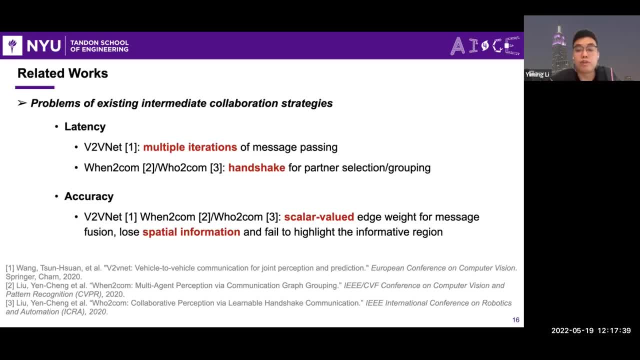 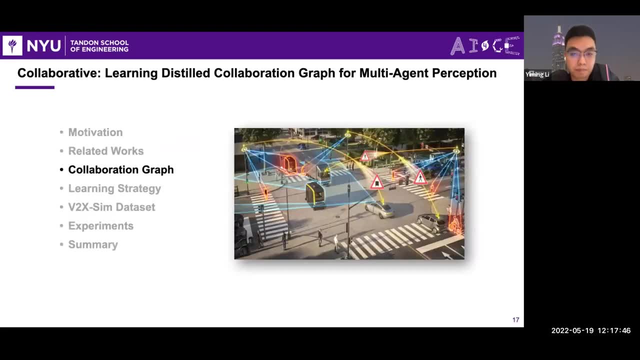 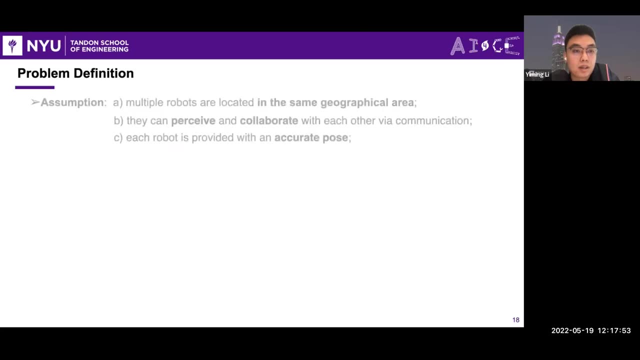 The other agent's message. So this can not highlight the information range or repress the noisy range. And now let me start with our, let me introduce our method. And the problem definition is that we assume multiple robots are located in the same area. 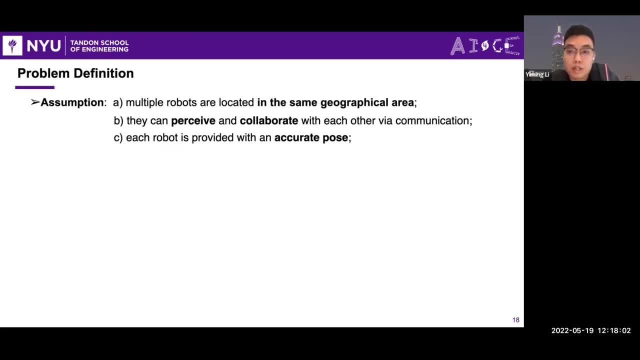 and each robot can proceed and also collaborate with each other via communication, And each robot is provided with an accurate pose, So so the robot can know where exactly they are, And our goal is now, given a certain communication bandwidth, we want to maximize the perception capability. 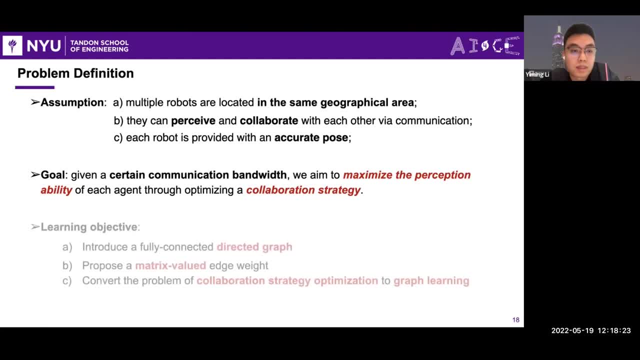 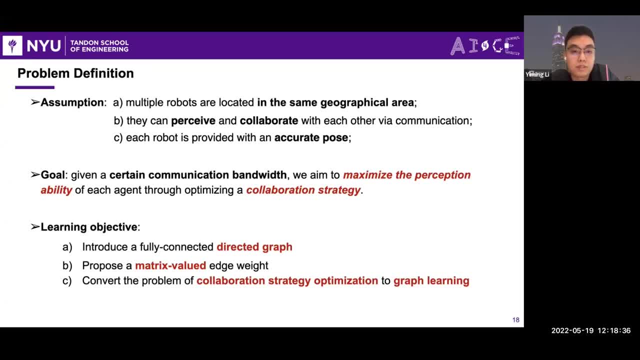 which is to model the collaboration among different agents. We propose some matrix value data, 80, eight, and then this head way, it's in this, into it It can highlight the information breach, For example, agents. one cannot see some kind of 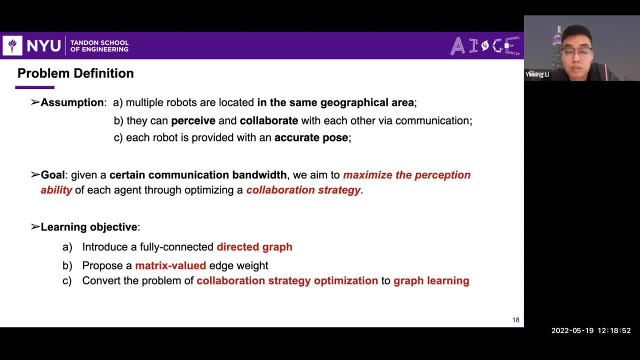 cannot see some cheek, so it's because some occlusion reasons. However, the agent two can just perceive such kind of range very well, so that it could highlight such kind of pixels. when we use the messages from agent two And now we convert, the problem. 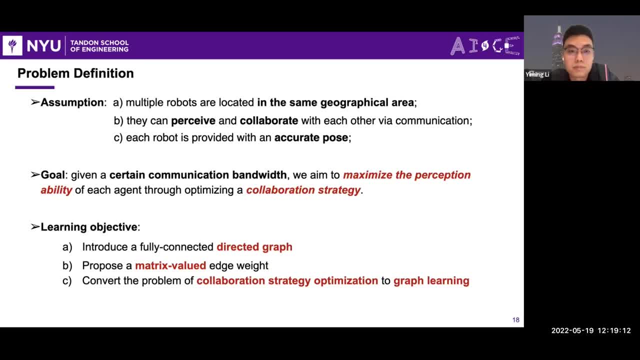 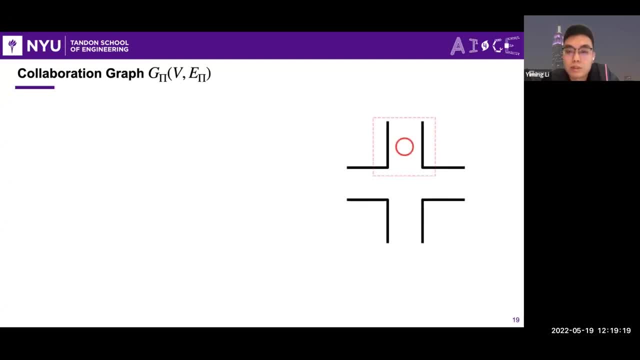 of collaboration strategy optimization to the graph learning problem. And now let me introduce our collaborative graph. Assume that we have multiple robots and, due to the limited sensing capability of each robot, each agent can only perceive a certain size, a certain range of its surrounding. 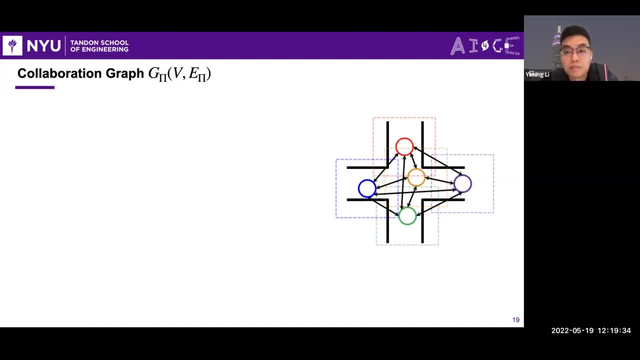 And we use the directed edge and which is bi-directional, to model the collaboration And also our graph is fully connected And for each node, since we are focusing on intermediate collaboration, and each node has an intermediate feature map and here, which 32 by 32, denotes the spatial resolution. 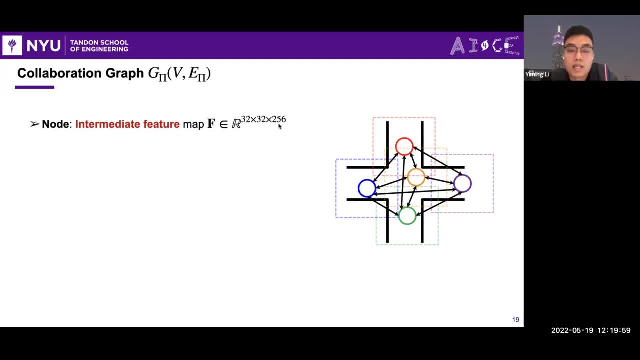 the lengths and the widths of these surrounding environment, And here 356 denotes the feature dimension. And also each node has its own six degree of freedom pose And our edge is directed and our edge width is matrix valued And our graph 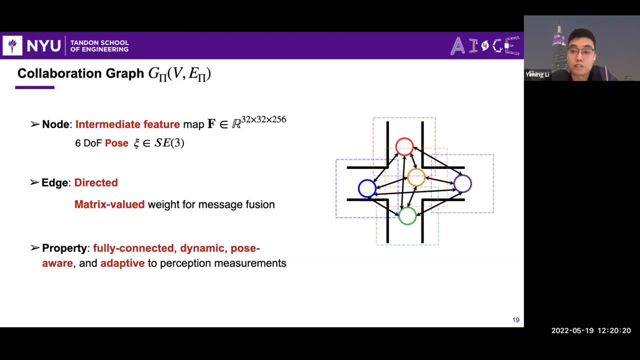 in summary, our graph is fully connected: dynamic because each vehicle is moving, So our graph is dynamic. And our graph is also post-aware because we know exactly the node, the nodes, location And also our graph. edge weight is adaptive to perceptive measurements. 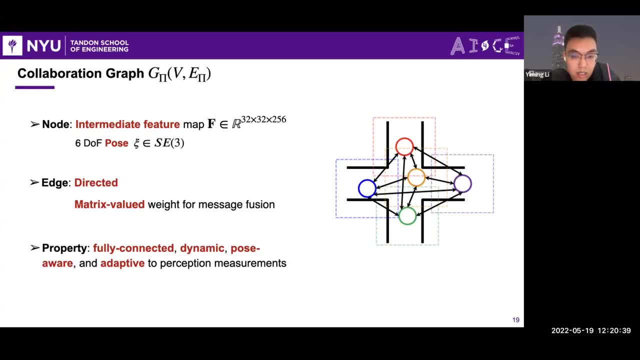 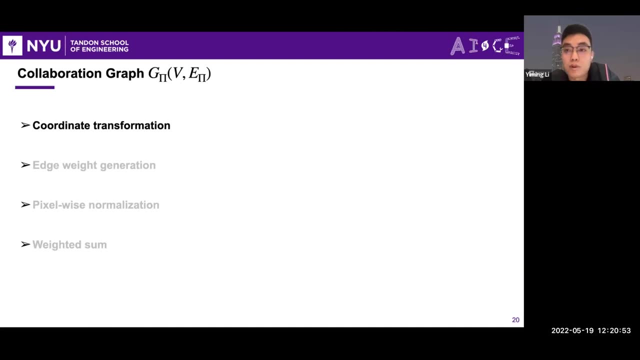 because, in different scenarios, the agent needs to highlight the different ranges, because it's running environment is changing right. Because so that we need to make our collaboration graph adaptive to the perceptive measurements. Now let me introduce our procedures for the collaboration graph. 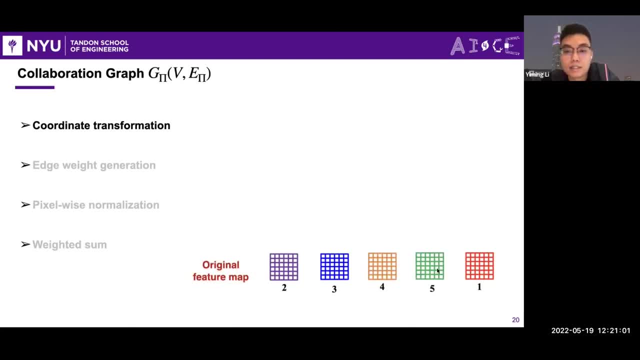 An image in that here agent one is an ego vehicle, And agent two to agent five are the neighboring agents. And now the agent one needs to aggregate the feature maps from its neighboring agents, And here this row denotes the original feature map. 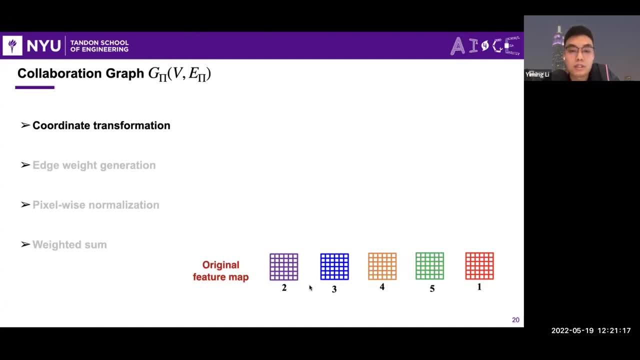 And the first step is coordinate transformation, because each agent has its own pose and its feature map is defined in its own coordinates, And so the first step is that we need to synchronize the coordinates right. So the first step is we synchronize the feature map. 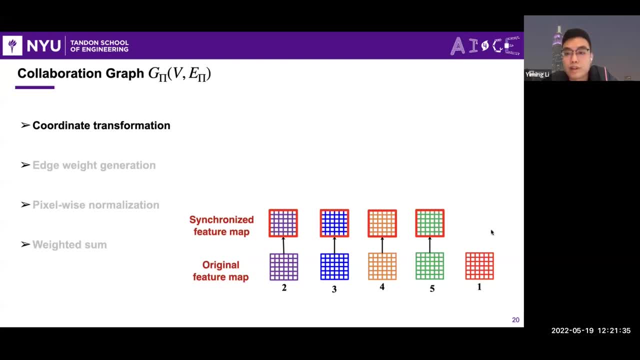 and make it these five feature maps in a unified coordinate which is defined in the agent to his coordinate And after feature map synchronization we need to generate the edge weight for each agent And to generate such kind of edge weight we use a convolutional neural network. 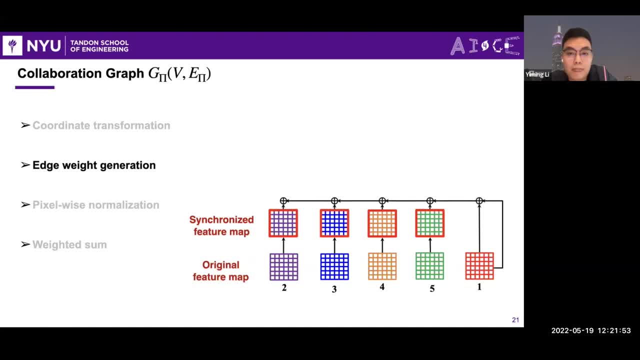 which is learnable during the training And our learnable edge weight generator takes the concatenation of the ego-agent feature maps with the neighboring agent's feature map and fit the concatenation of these two feature maps into a convolutional neural network and the output matrix And this matrix. 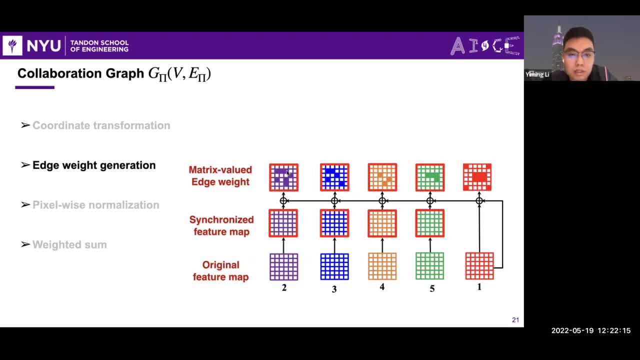 denotes the age rate And the pixels with higher value denotes that this pixel is very important because agent two can see some elements which cannot perceive agent one And for some pixels the agent two do not have measurements, then its pixels will have a lower importance score right. 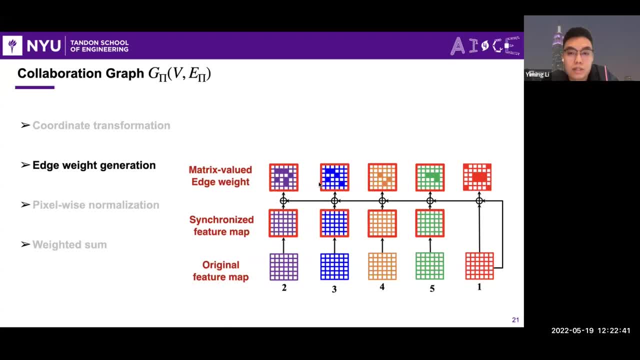 So through such kind of matrix-valued weight, our ego-agent could highlight the informative range while repressing the noisy range. And next step is pixel-wise normalization. because here we can see, this is the new pixel-wise normalization. The next step is pixel-wise. 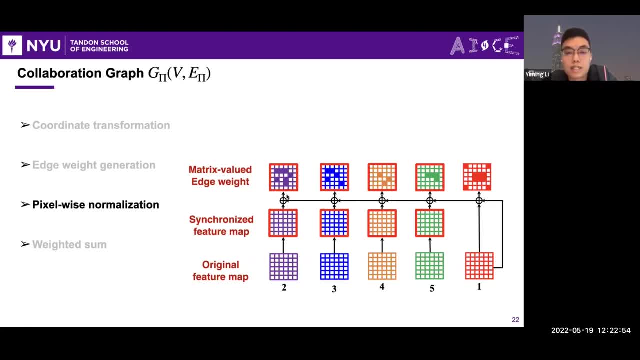 or the bias-based normalization of the pixel-wise samples versus the bias-based samples, Right. And the next step is pixel-wise normalization, because here we can see that the we have five feature maps and we want to conduct a witty sum of these five agent, five feature maps. 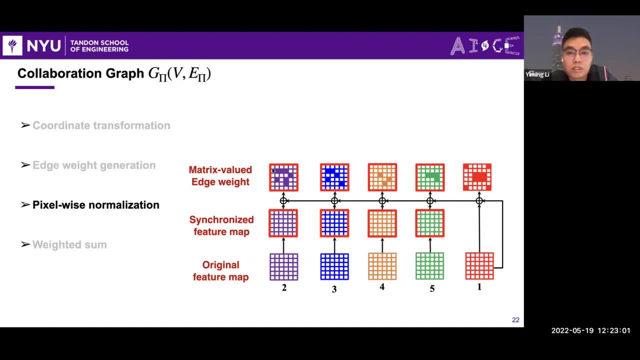 from five agents and for each pixel, for each pixel, it actually here each pixel denotes one spatial area at which is defined in the ego agents coordinates, and for each pixel we conduct a pixel-wise normalization and so that finally, we can conduct, implement a weighted sum of all these. 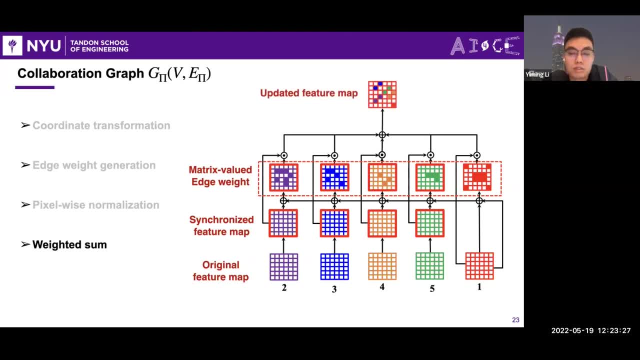 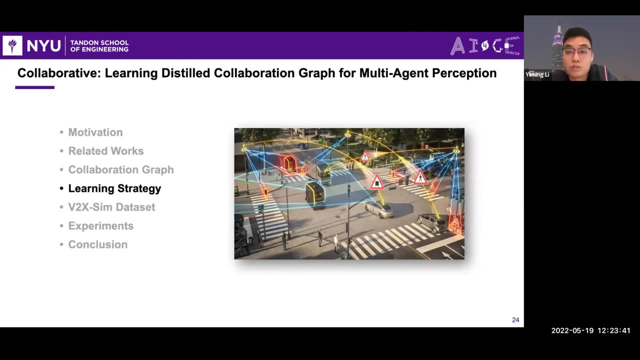 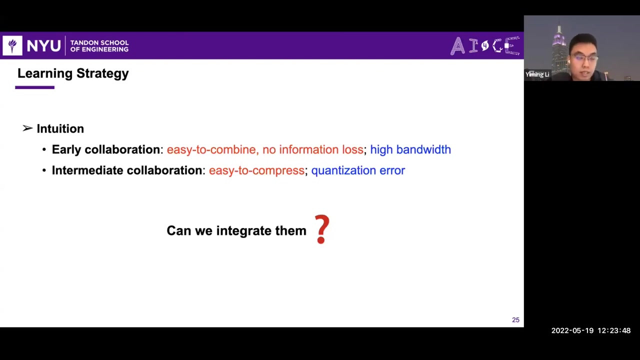 five feature maps to get to the final updated feature maps. so through such kind of matrix valued weight, we can highlight the different pixels with different importance scores. so now let me introduce our learning strategy. the intuition of our learning strategy is that for early collaboration which is based on the input, the raw data input. 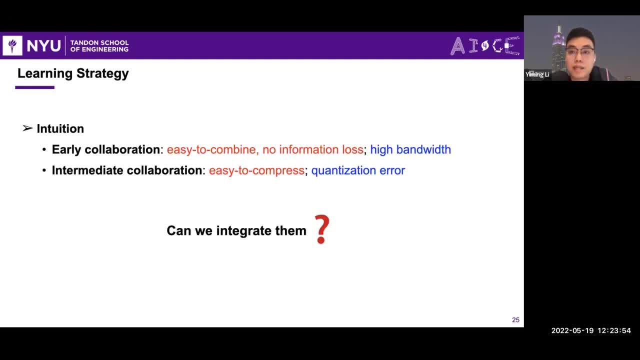 fusion. it bandwidth is high. however, its performance is better because there is no information loss and for the intermediate collaboration. although the feature map is easy to compress, however, there are several convolutional layers which will introduce the quantization errors. so our intuition is that: can we combine these two methods into a unified framework so that we can 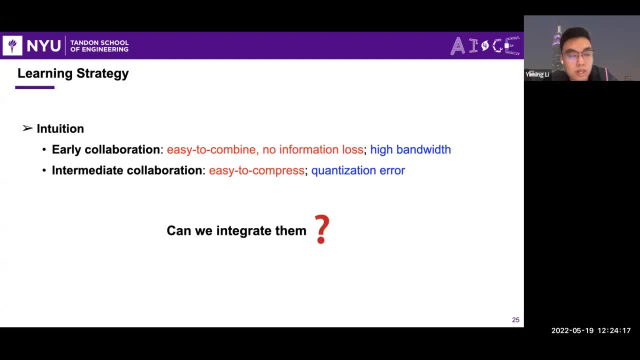 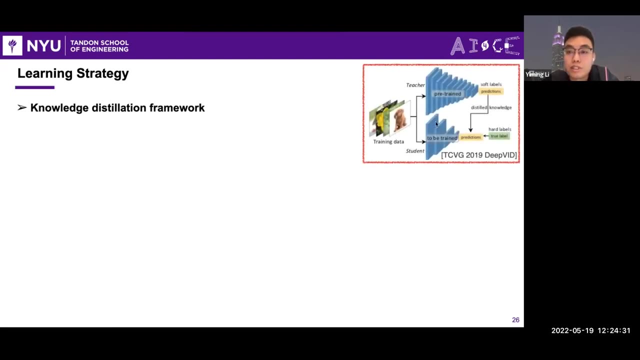 we can have both of these two advantages while repress repress their own disadvantages and we utilize knowledge distillation framework. and knowledge distillation framework is widely used technique in machine learning and computer vision community and the basic idea is that you have a teacher model which has a lot of parameters, which is which has more parameters. 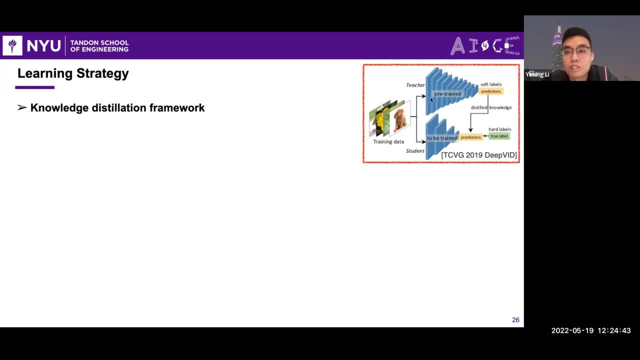 than the student network. and then during training you firstly train such kind of teacher model for a teacher network with more parameters and this will introduce a high, high computation. but after training such kind of teacher network and we will fix the parameters of teacher networks and then start training the student network, which is more lightweight, and so the student network. 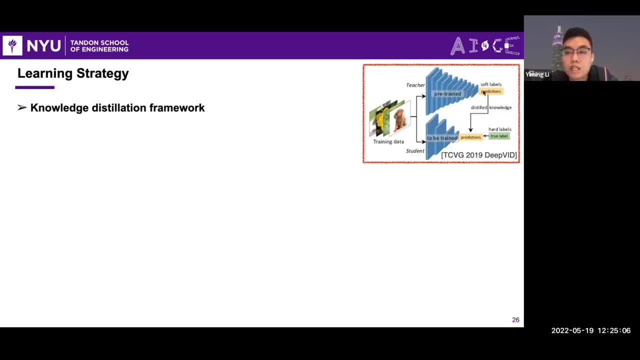 could, could imitate the behaviors, the output of the teacher network, in addition to the ground truth labels. so we, we use the ideas of knowledge iteration, but we are. we are a little bit different and here our teacher is our teacher student network has the same skill and they have same parameters, same numbers of. 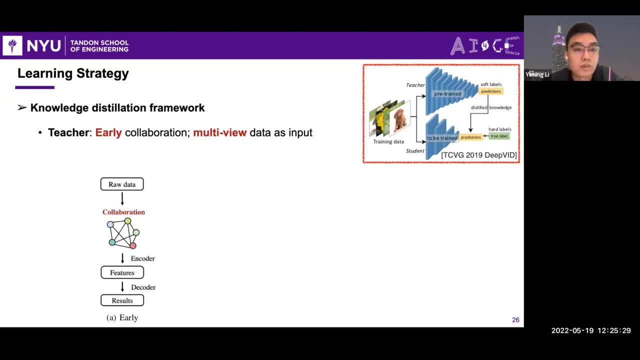 parameters. however, the input is different and the teacher networks is based on early collaboration, which they just fuse the raw data starting from the input right, and our network has no information loss, so its performance is the best and our student network is based on the uh intermediate collaboration. you can see that here we first use a uh, use a encoder to 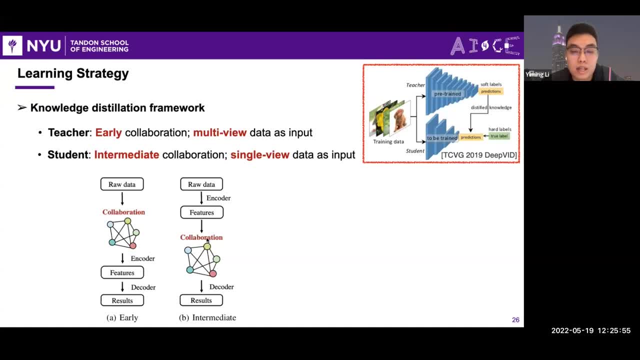 extract its features and then we will implement collaboration uh in the feature maps, in the feature space, and so our student network is based on single data uh, single data input. while we implement intermediate collaboration and during training, we will use the, our teacher network, which is based on early collaboration, uh to guide the training of our 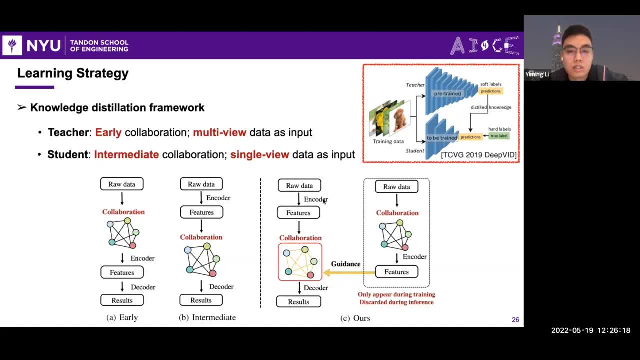 intermediate collaboration so that, OK, although we do not implement the intermediate, although we do not implement raw data fusion, but we can let our intermediate fusion-based methods to imitate, to try to approach the performance of the teacher's network which is based on the early fusion. 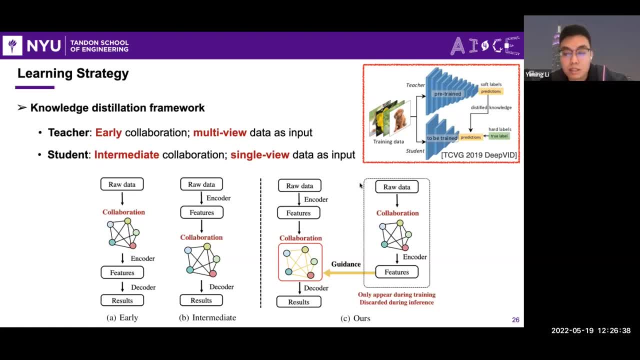 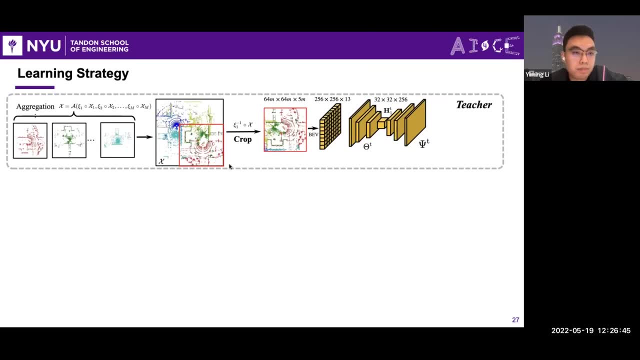 That's the basic intuition and the technique to achieve this. Now let's see a detailed framework Here. you can see that here the top figure denotes the teacher's network and it takes the multi-view data as input. You can see that. 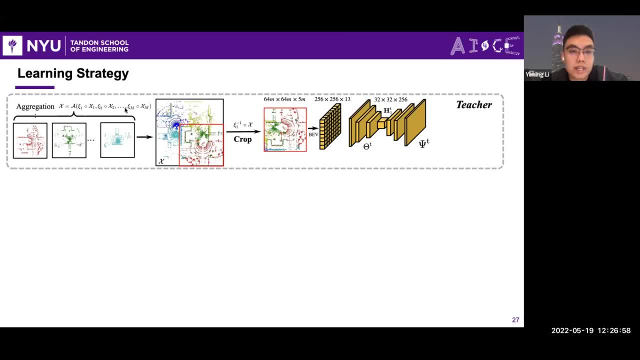 we firstly aggregate all these point clouds from different vehicles and we get multi-view data, and then we can input the multi-view data into our teacher networks. And here please note that here this operation denotes the bird's eye view map voxelization For a given point cloud, because it is just 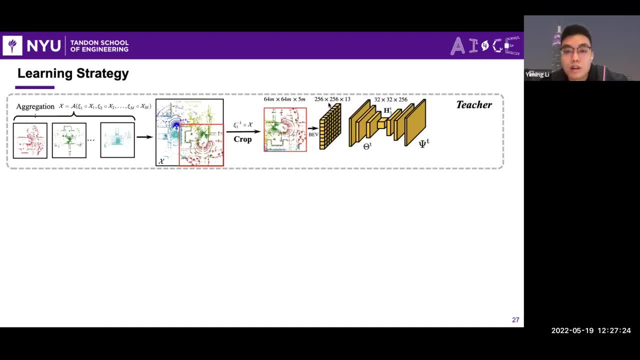 a set of points. we need to make it into a regular voxel grid. We just divide the space into several voxel grids and we now start to account the numbers of the points in different grids If the grid is occupied by at least one point. 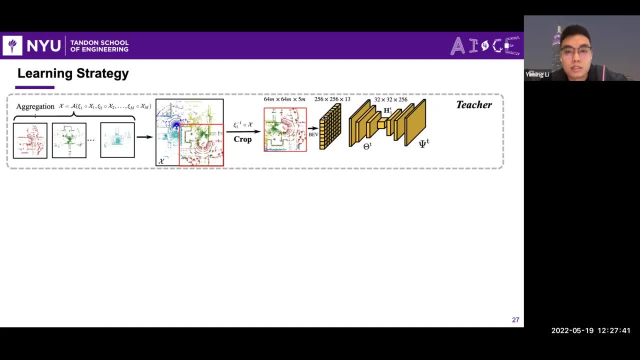 then it is equipped with one And otherwise it is equipped with zero. So this BEV representation is just some binary pseudo image, and so that we can use the two-D convolutional neural network to process such kind feature map, BEV feature map. 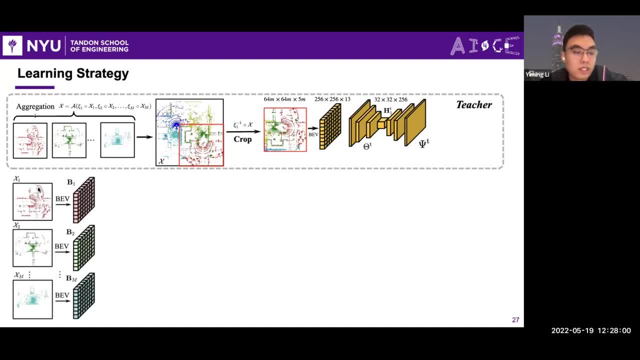 For our Walkthrough Network. you can see that for each individual, individual viewpoint, we first implemented Bird side-view voxelization to make it as the pseudo image, and then we we input them into our encoder separately and we can get the corresponding feature maps. 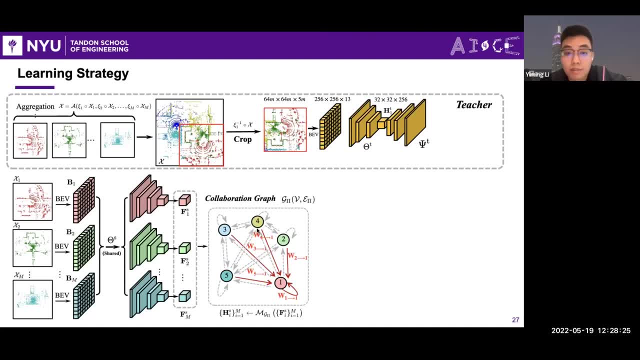 And then we use our collaboration graph, which is a fully connected directed graph, to do the collaboration And after such kind of information propagation we can get our updated feature maps. And then we will fit our updated feature maps into our decoder to get the final results. 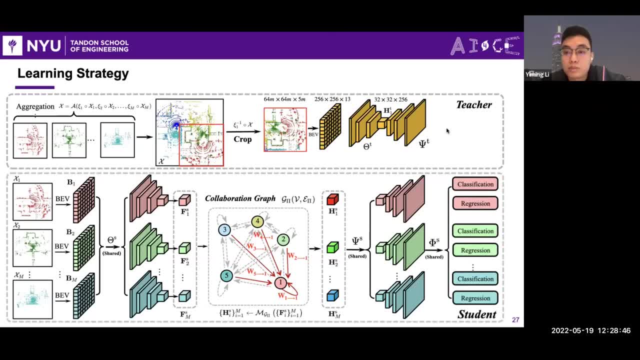 And this is our student network. So during training we first train our teacher network and then we will use knowledge distillation to minimize the difference between the intermediate feature maps from both teacher networks and student networks. Basically, we just try to let our students 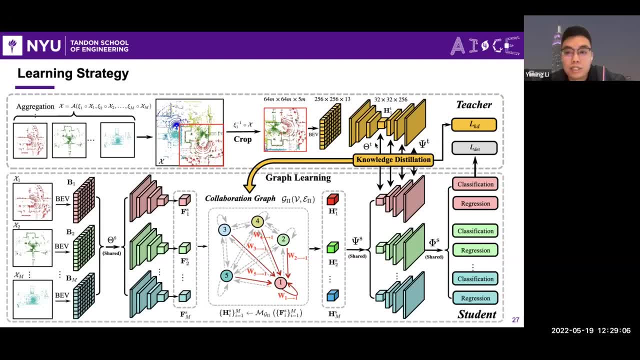 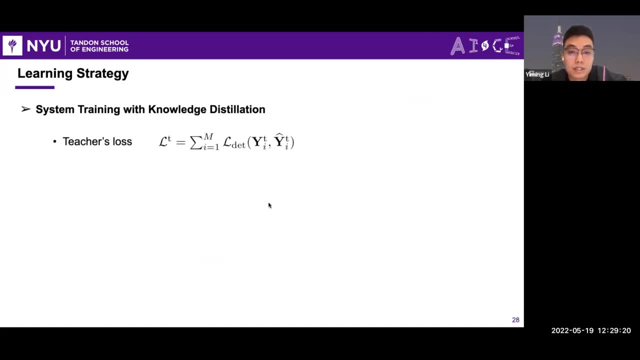 to approach the performance of the teacher networks, And so this kind of training technique could guide the. our collaboration graphs. learning And our teacher's loss is just a detection loss, which includes the classification and the regression loss of the bounding box, And our student loss not only includes the detection loss. 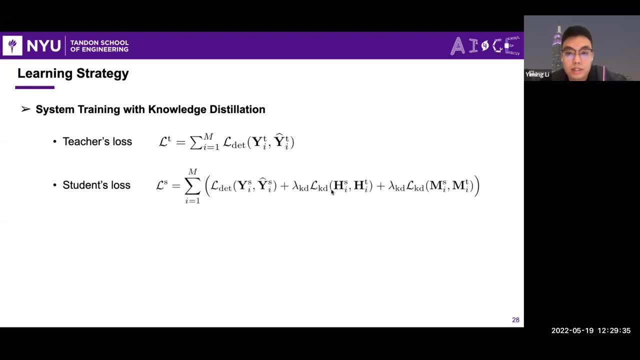 but also we have a knowledge distillation, the KD loss here And we will minimize- And here we can see that the KD loss is just a detection loss. And we can see that the KD loss is just a detection loss And we can see that the KD loss is just a detection loss. 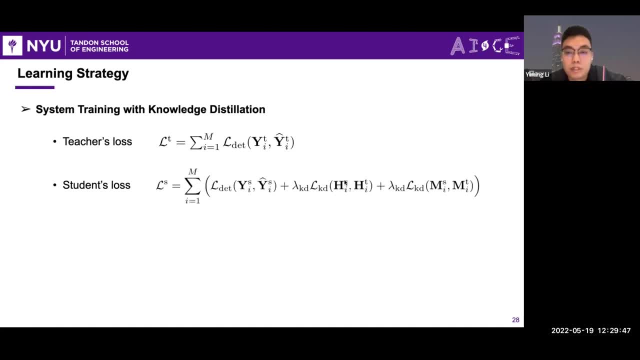 And we try to minimize the intermediate feature maps between the students and the teachers And the KD loss is just. we just use the KL divergence to mirror the difference between these two feature maps And I will not introduce the details of this loss function. 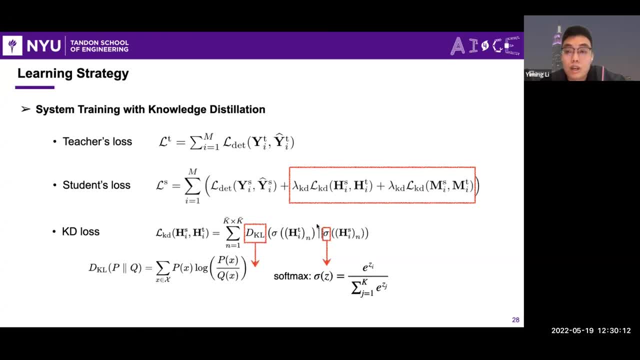 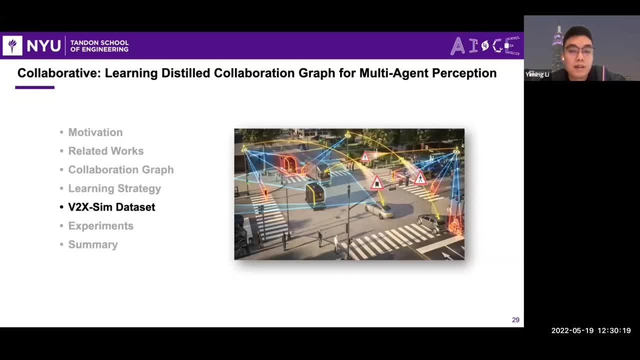 but the basic idea is that we try to let the student network to approach the performance of the teacher. Okay, that's our method. We firstly introduce our collaboration graph, which is a fully connected directed graph with a matrix-validate rate, And then we introduce the learning strategy during training. 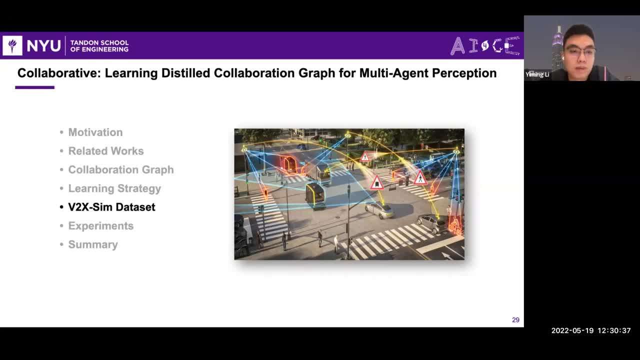 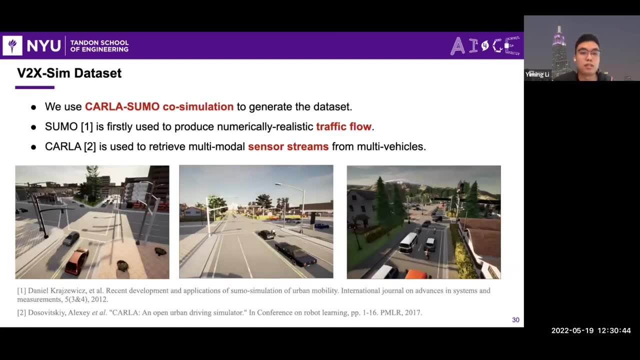 to learn such a collaboration graph And now let me introduce the experiments. And to verify our method, we need a dataset. However, there are no real-world datasets for the vehicle-to-vehicle collaboration, vehicle-to-vehicle perception research, So we use a KLR sumo correlation to generate a dataset. 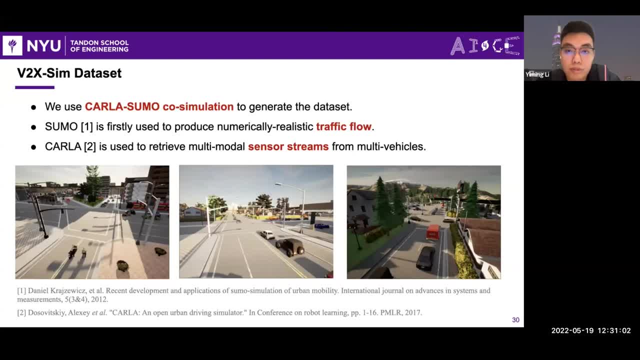 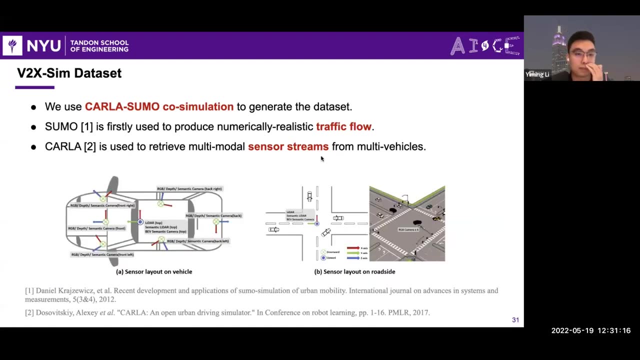 and we use a traffic simulator, sumo, to produce a numerically-realistic traffic flow. And then we use KLR to retrieve the sensor streams from multiple vehicles at the same intersection. And also we attach- not only attach sensors onto each vehicles, and we also 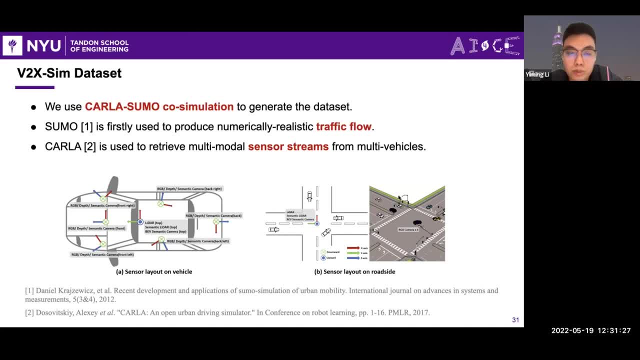 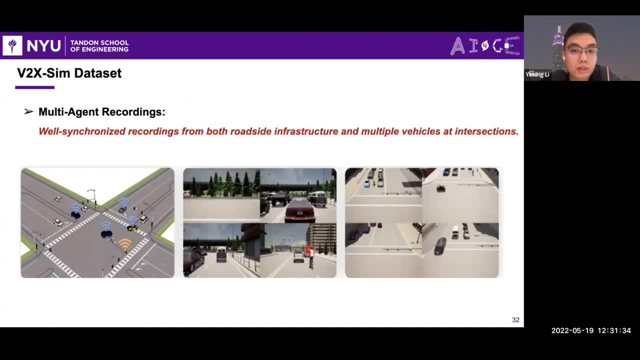 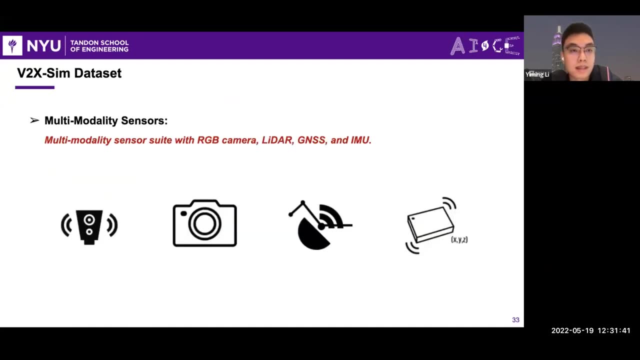 attach sensors on the roadside unit to achieve both vehicle to vehicle and vehicle to intersection collaborative perception. So our dataset has multi-unit recordings from both vehicle and the roadside unit And we have multi-modality sensors including RGB camera and 3D, LiDAR and GPS and IMU And we provide semantic labels. 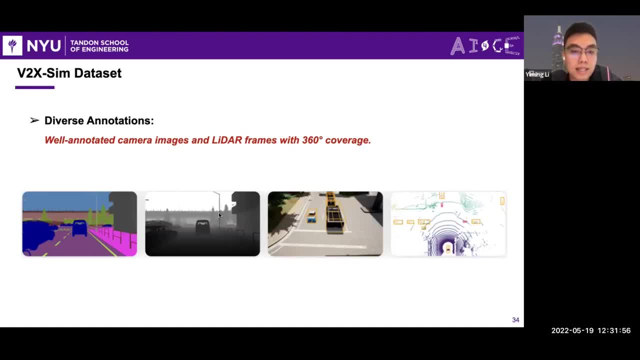 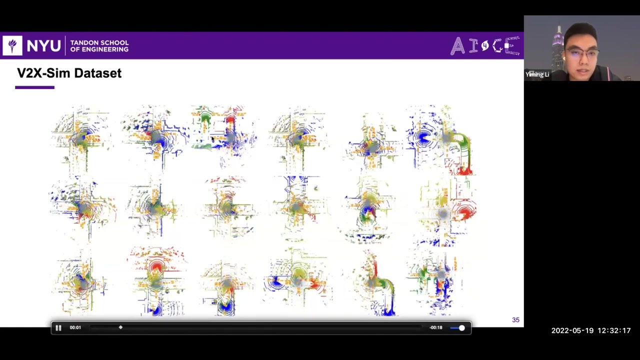 3D bounding boxes and ground-truth steps to enable the perception research, because we need some ground-truth labels to supervise the perception models, training And in simulation. it is quite cheap to obtain such kind of ground-truths And this video shows our dataset in bird's-eye view. 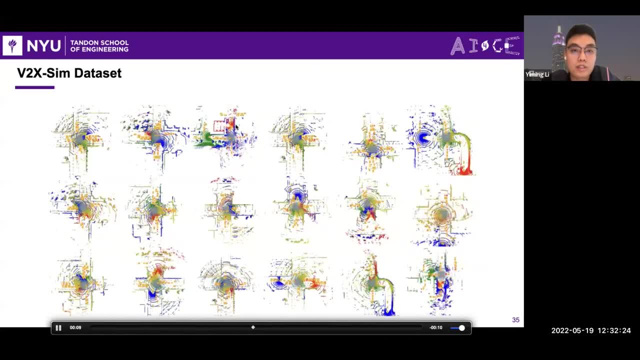 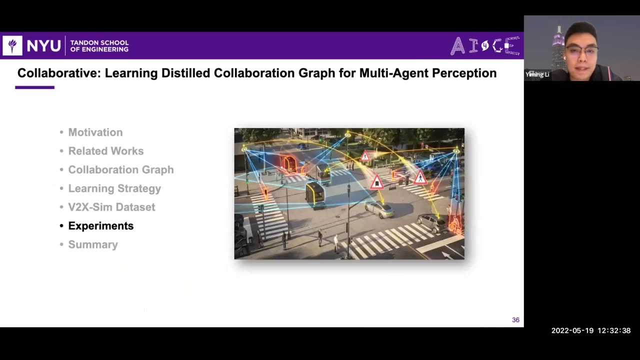 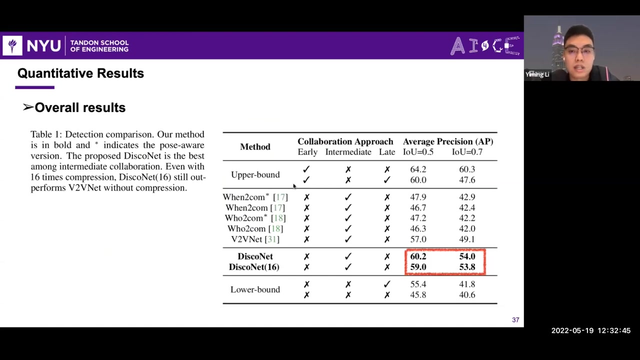 and in the top-down view, And each color denotes the environments from different vehicles And the orange boxes denotes the moving dynamic vehicles. at this intersection And after generating such kind of dataset, we can verify our results, verify our method And our method learning. 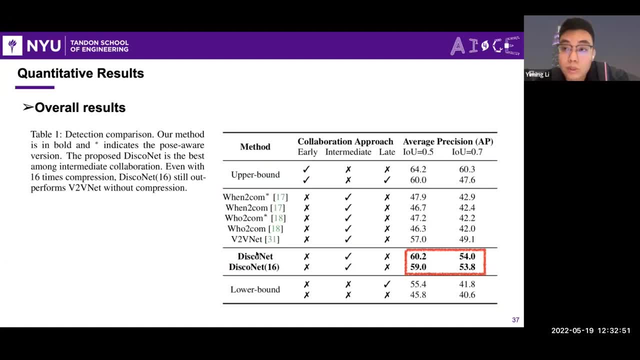 distilled collaboration graph, which is, which is named Disconet. You can see that our method achieves the best performance compared to other intermediate methods And here, when to come, and between that, we have better performance than its intermediate collaboration methods And we can. we also have, our method, can also try to approach. 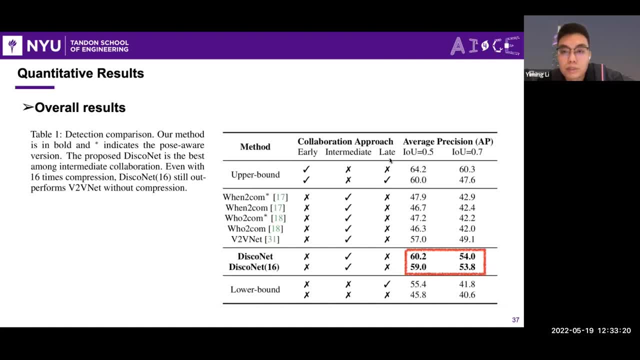 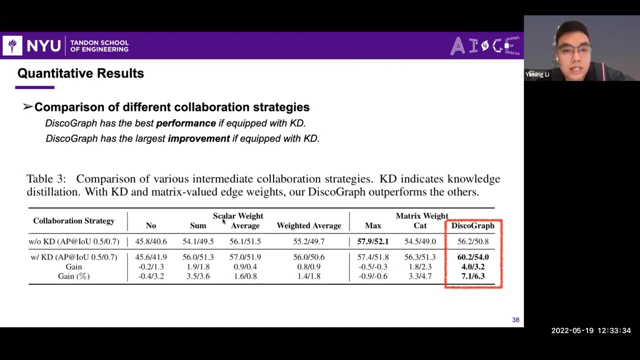 the performance of the upper bound, which is based on the early collaboration. But there is still. there is still a space for the improvement And compared to other different collaboration strategies, like we can just sum the feature maps from different agents or we can use maximum collaboration or the concatenation. 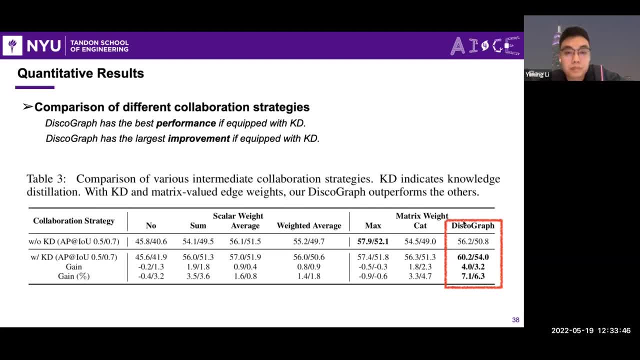 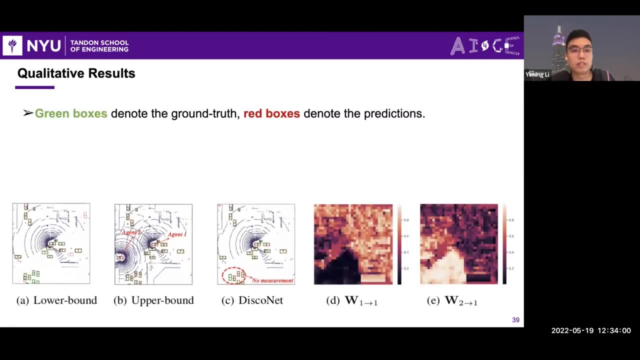 collaboration. we have the best performance when we equipped with knowledge distillation framework, And also we have the largest improvement if equipped with knowledge distillation. And now let me show you some interesting visualization results. And here this figure: in this figure, the green boxes, you know. 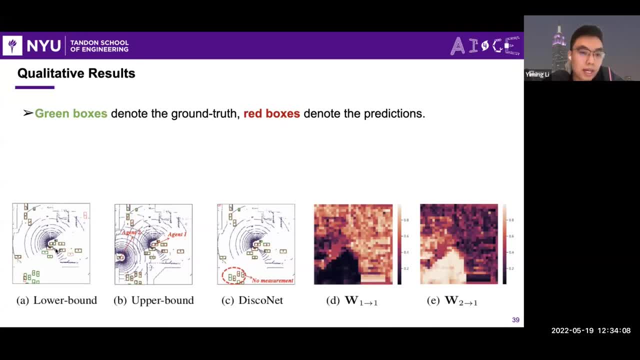 the ground truth box and the red box. it denotes the predictions. You can see that for the lower bound, which they are, there is no collaboration, And the in the left bottom corner, since there is no measurements for this vehicle. right so the vehicle. 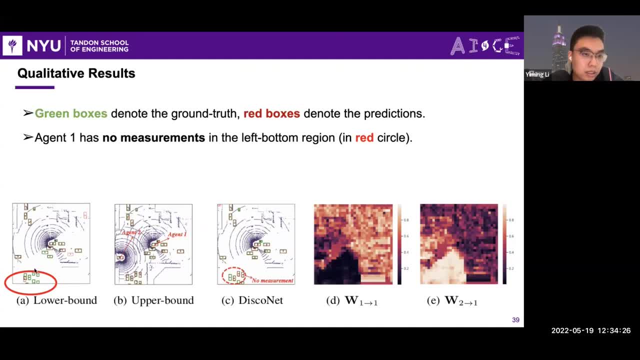 can hardly perceive the these, these bounding boxes, right, because it has no measurements. So it is impossible for the agent, for the algorithm to calculate the, to compute the bounding box at that, at that corner. And here now we have another agent, agent two. 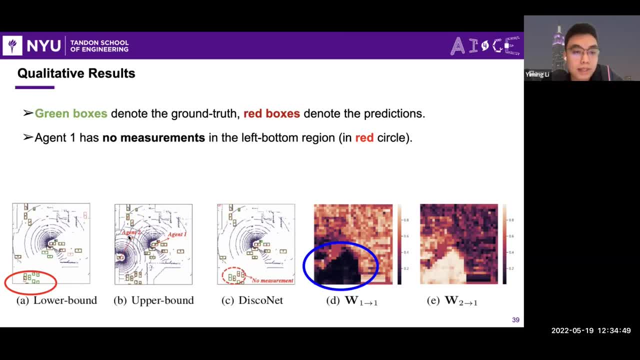 right. Agent one needs to aggregate the information from agent two, And agent two can perceive this range well, You can see that it has a lot of measurements located in this, in this corner, In this yellow circle right, And then in our, let's say our, age weight. And for the age weight from agent one, 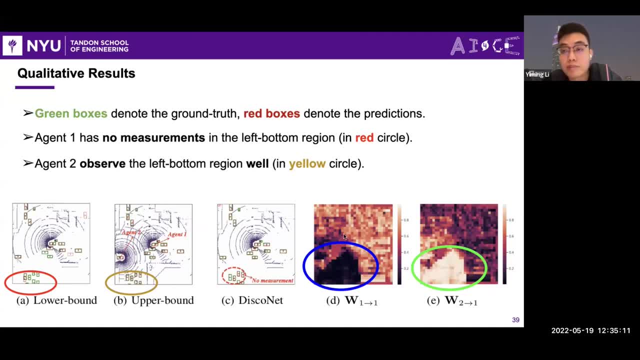 right agent, one which means it's self-age. during weighted sum fusion, the ego agent also needs to weight its own message. So during its in its self-age weight, it will lower its confidence right Here: the brighter. the darker color denotes the lower value, and brighter. 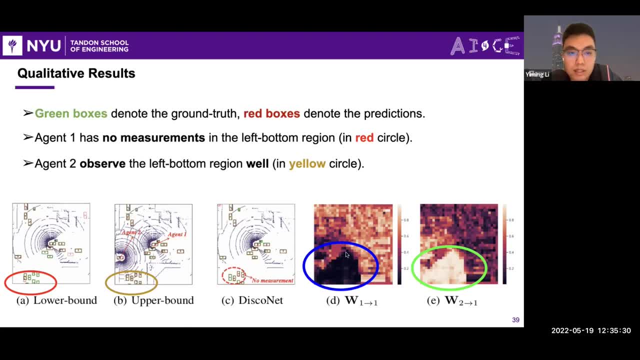 color denotes the higher value. You can say that because agent one cannot see the left bottom corner and it will lower its confidence in this range And for the age weight from agent two to agent one, which means that the agent one needs to fuse the agent two's. 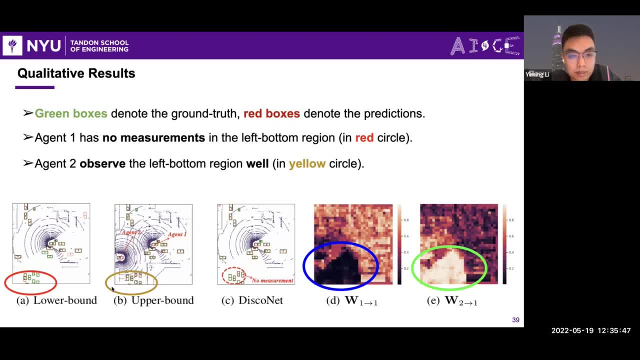 information. right, Because agent two can see such kind of range And so the in the age weight it will highlight these pixels, these pixels, You can see that this spatial range is complementary And it can provide complementary information for agent one. right, So that? 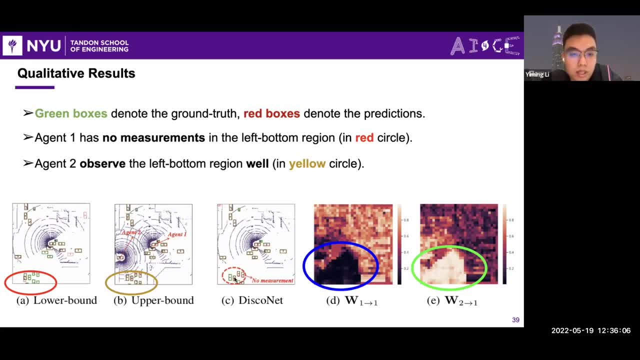 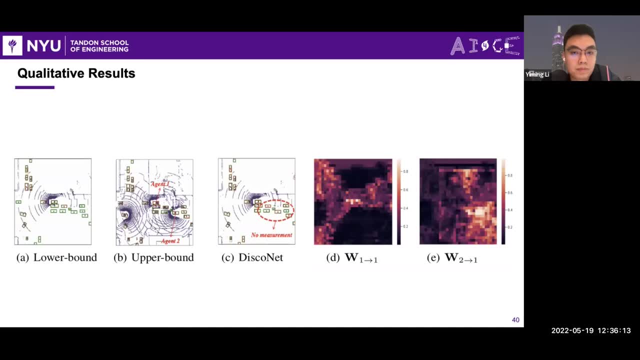 after collaboration. you can see that our method can perceive several of these four bunny boxes located in the left bottom corner. And here is another visualization example. And you can see that in the top part the ego vehicle cannot perceive any measurements due to the occlusion And so in its self-age weight. 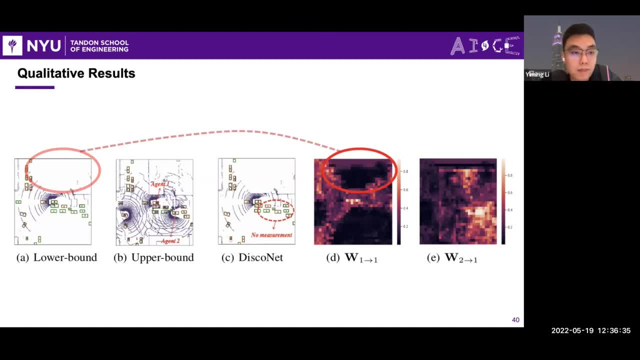 it will lower the confidence at this part. Similarly, the bottom part in the bottom part agent also has no measurements. So it will also reduce its confidence values in these pixels. And agent two has good observations in this green circle. So for the agent for the age weight from agent two to agent one it can. 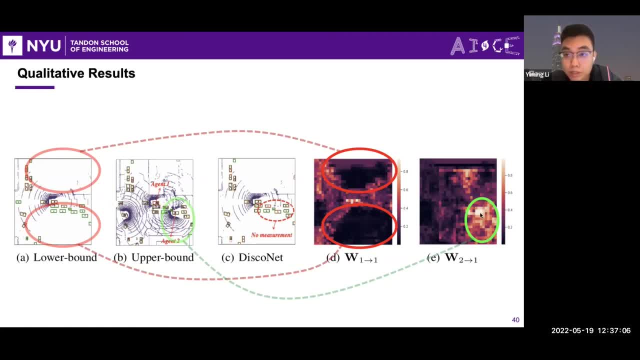 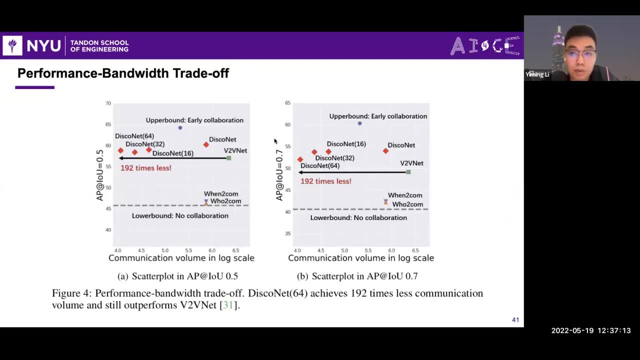 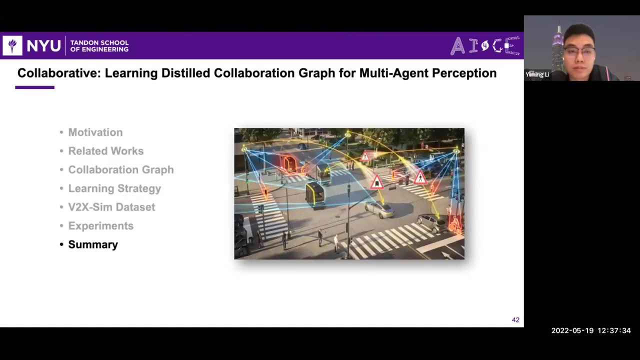 highlight the corresponding pixels And we also implement compression, dimensionality reduction experiments. We try to further compress the feature maps of the intermediate representation And we find that our method can achieve a better performance: bandwidth trade-off. Okay, that's for our first part, collaborative perception. 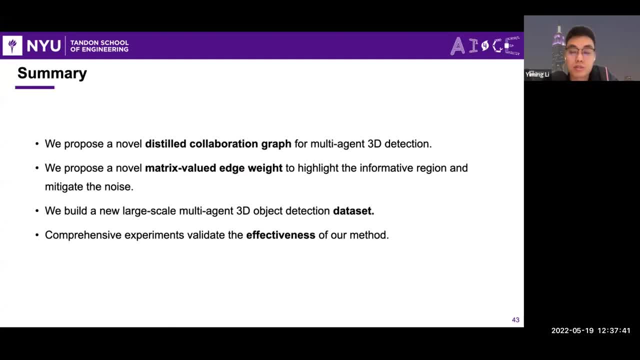 And, in summary, we propose a novel distilled collaboration graph for multi-agent 3D detection And in this graph we use the matrix-validated way to highlight the informative range and also mitigate the noisy range. And we also propose a new data set with color-smoke simulation. 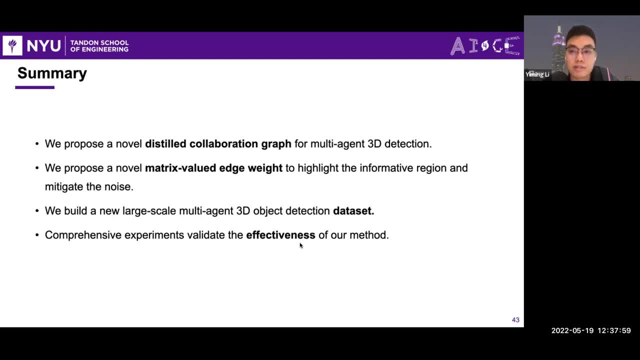 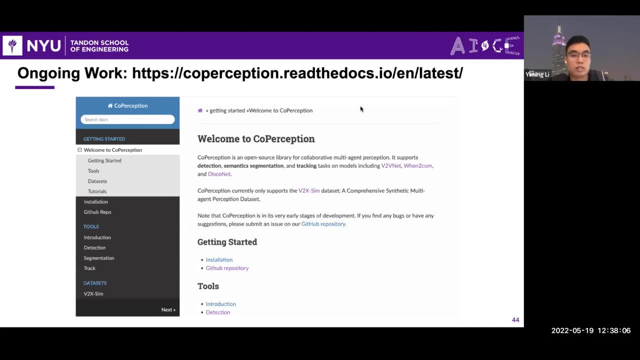 And we conduct the experiments to validate the effectiveness of our method, And currently our ongoing work includes developing an open-source library for collaborative multi-agent perception And in this library we try to offer some tutorials to implement different collaborative strategies and also with different 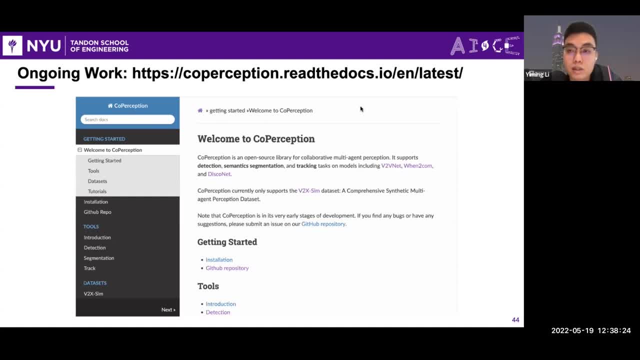 single-agent detection backbones And we also include. we also try to include more tasks like more perception tasks like semantic segmentation and object tracking, And we try to make it an open-source library so that researchers with with interest in these areas can utilize our library. 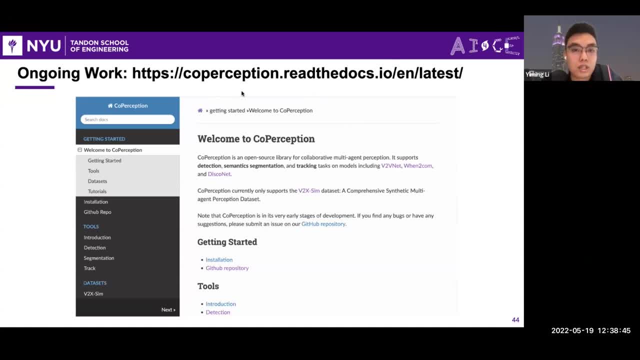 And if you are interested and feel free to, feel free to check our website and you can just Google core perception and try to find the library website And we are still still working on it. So it's so this, the current version, might not be. 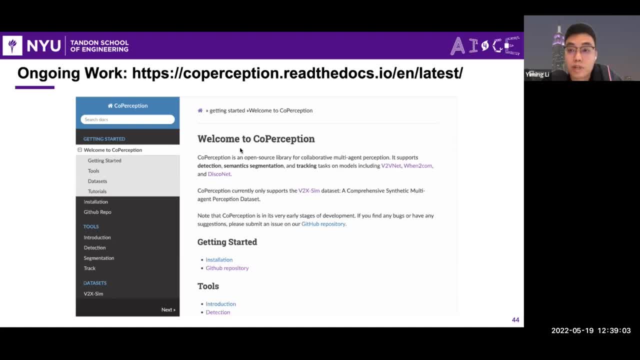 complete, but we will try to continue to improve our tutorial. And also, if you have interest in developing such kind of tutorial and library with us, you can also email me or email my advisor, Professor Chen Fen, and we can talk about that definitely. 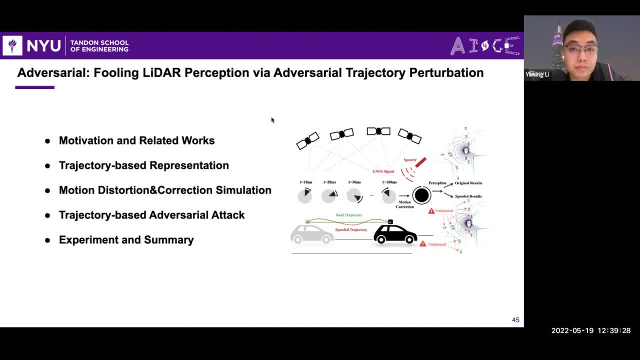 Yeah, thanks, John. Okay, so now let me introduce the second part: adversarial perception. In this work we propose to propose a new structure-based adversarial attack framework And we try to review and overlook vulnerability which lies in the motion compensation process. 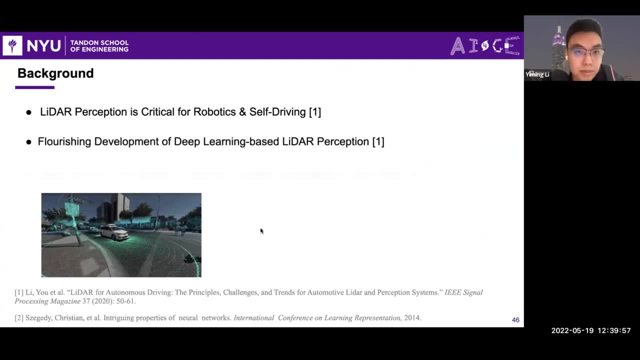 And for the background here, the LIDAR perception is very critical for self-driving And this is the we have. we have introduced this before and there are some, many kinds of deep learning based LIDAR perception algorithms have been proposed. 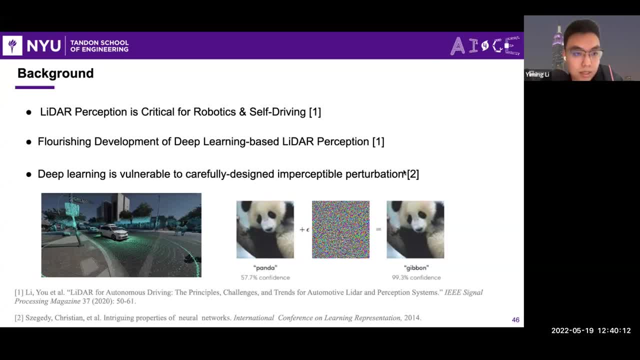 And the third. the third part is is that deep learning is vulnerable to carefully designing perceptive perturbation. And this is quite interesting in deep learning communities because for the for for for deep learning models, it is vulnerable to some carefully optimized, which is. 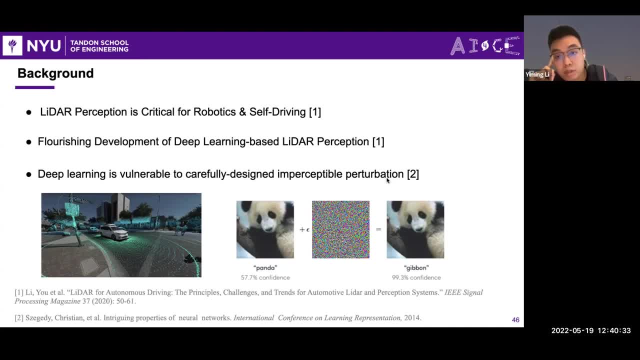 which can attack the, which can actually achieve adversarial attacks of the corresponding deep learning models, For example in a 2D image domain. here is the, here is an object, and while we optimize some kind of imperceptible adversarial noise using gradient-based methods, 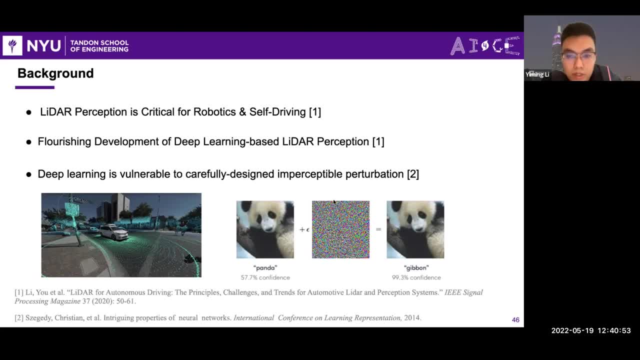 and when the when this image is edited with, with, with such kind of noise, although it still looks like a panda for the human eyes, but for the deep learning algorithms it will misclassify the animal right. So this is quite interesting in the deep learning community. 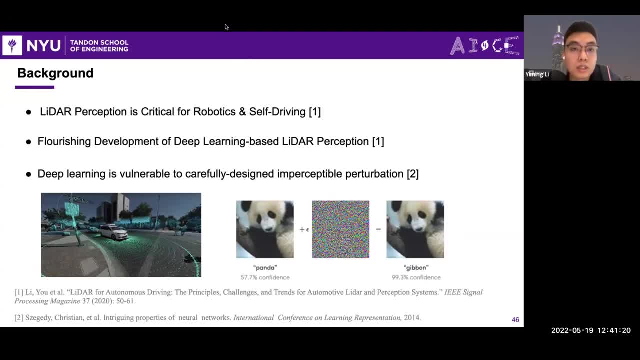 And I see a question in the chat box. Yeah, we can get to it now or at the Q&A, but the question is asking you if you could highlight a few points on how to deal with multi-sensors of different modalities with varied frame rates. 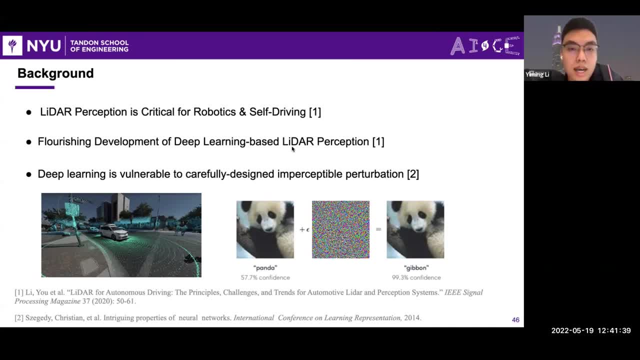 Yeah, that's a very nice question And currently we are focusing on the single modality, private perception, and we focus on the 3D point cloud modality And in the next step we try to involve more modalities like cameras, right. 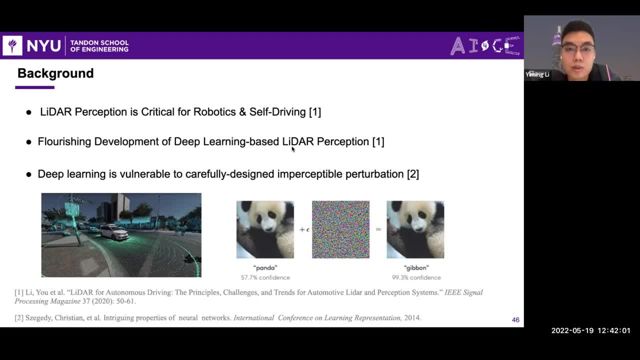 And I think that's a very interesting topic, But currently we just focus on the single modality: collaborative perception. Yes, if you want to add more modalities, the system will become more complex and it requires more investigations and we need to think about it. 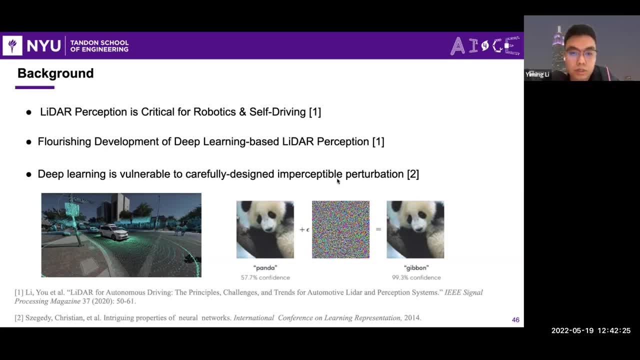 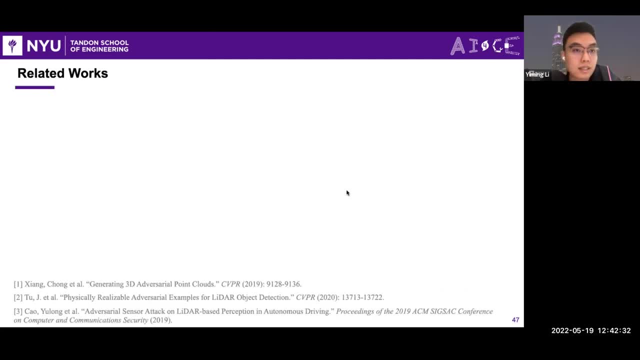 Yes, let me continue, Okay. So I think that's a very interesting question, And I think that's a very interesting topic, And I think that's a very interesting topic to discuss. And so the researchers have proposed various algorithms around the adversarial learning. 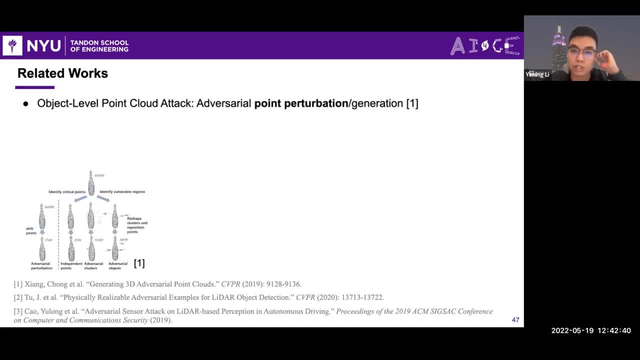 in computer vision And for the 3D computer vision. some researchers proposed some frameworks to attack the point cloud, point cloud classifier. For example, they proposed adversarial point perturbation or generation to to make the point cloud classifier misclassify the corresponding objects. 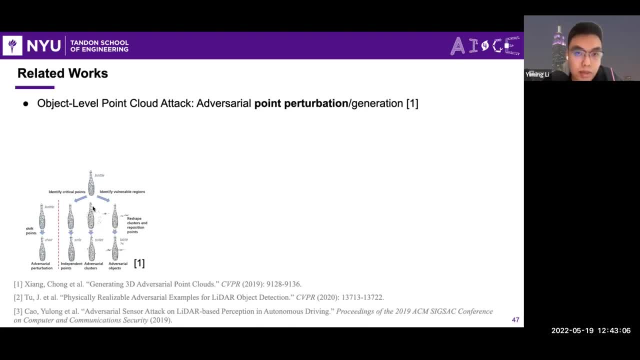 And basically its idea is that try to use some very imperceptible perturbation, apply some imperceptible perturbation onto several key points and then the deep learning models will misclassify the corresponding object. And also, very interestingly, the Uber autonomous driving group. 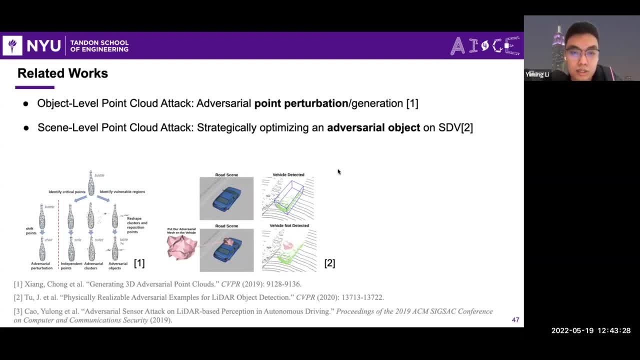 they have proposed some scene-level point cloud attacker. They carefully designed some adversarial object which can be put on the top of the corresponding vehicles and this vehicle could be invisible to the deep learning-based 3D black detection. And also there are some sensor attack. 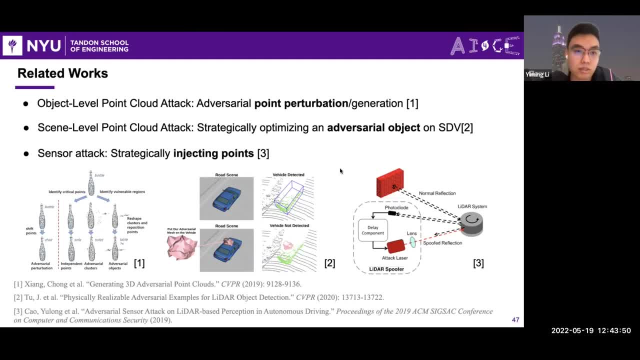 and they utilize some physical-based methods to strategically inject the points into the scene. For example, they just inject some points which are located in the critical parts, for example, which is in front of the car, so that the cars will sort that there is an object. 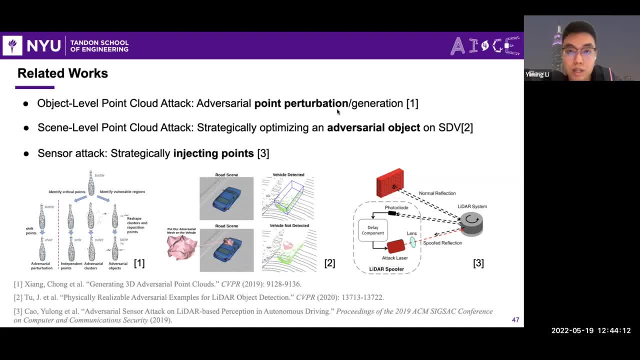 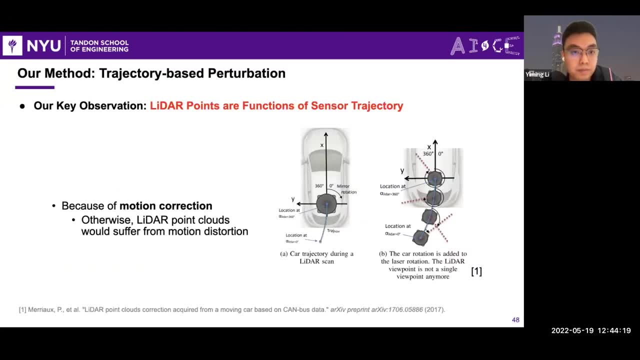 in front of it, right, And so that it will have some dangerous driving behaviors which can hurt the safety of the passenger. And our method is that? different from the previous methods which try to manipulate the point, each individual point's coordinate, we try to propose trajectory-based perturbation method. 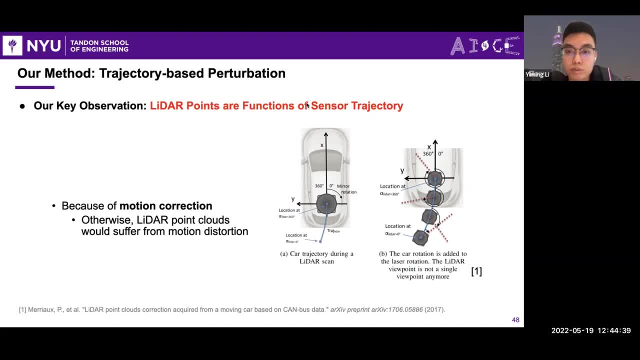 And our key observation is: LiDAR points are functions of sensor trajectory. You can see that in this vehicle it illustrates such kind of motion distortion scenarios because when the LiDAR is rotating to capture the measurements of different spatial ranges, the car is still moving right. 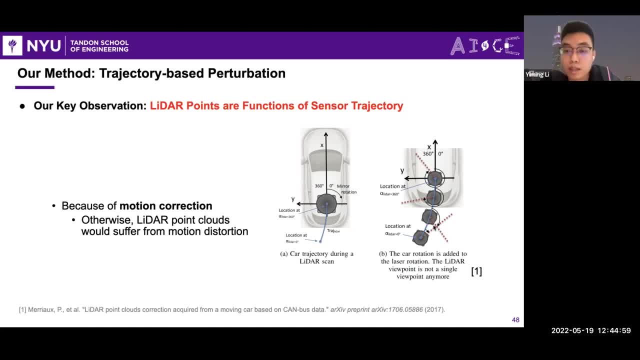 So the sensor attached onto the car is also still moving so that the different measurements are captured actually at different locations. And, finally, you need to use your location information such as: basically, the localization systems is based on the GPS system. 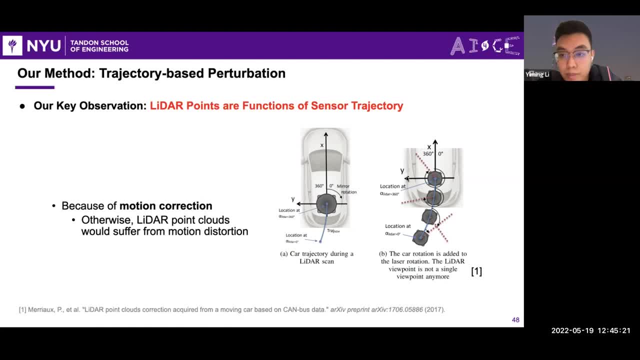 and you need to utilize that kind of GPS trajectory to make all these measurements. you know unified coordinates so that it can remove such kind of motion distortion And then most methods focusing on the distortion-free point cloud, which means that it does treat the same level point cloud. 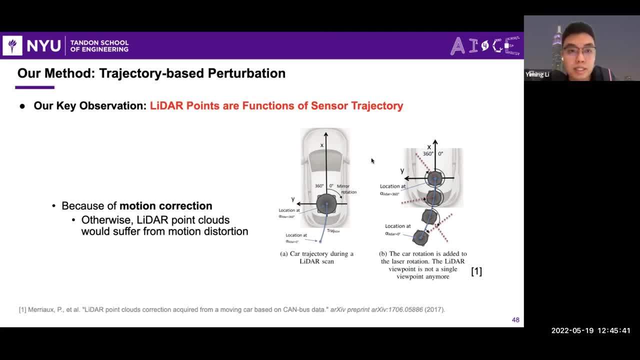 as the functions of the coordinate. but our observation is that actually the LiDAR points can be treated as a differential functions of the sensor trajectory. And here here P denotes a set of points Which is covers the full view, full 360 degree view. 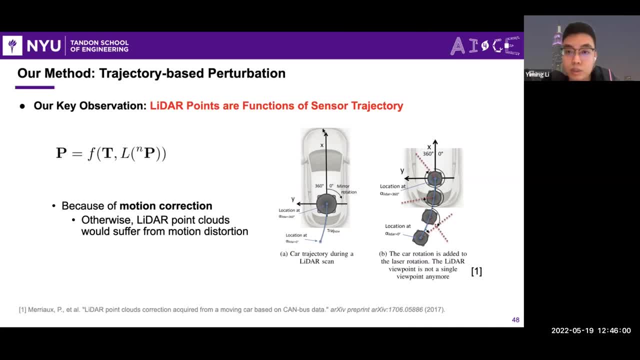 And this a full view, is divided into different sectors, which is denoted by, which means that they are captured at different locations, And here the T denotes a vehicle trajectory and it is a set of the transformation matrix, And here PN denotes a corresponding LiDAR packet. 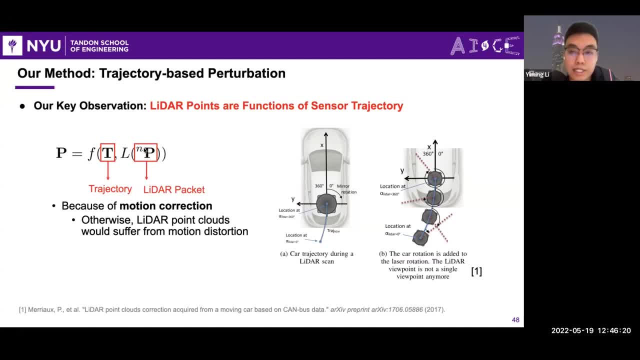 And so this function means that for each LiDAR packet it's captured at a certain trajectory point, so that when we aggregate all these points, all these points captured at different locations, we can have a final full view point cloud right. 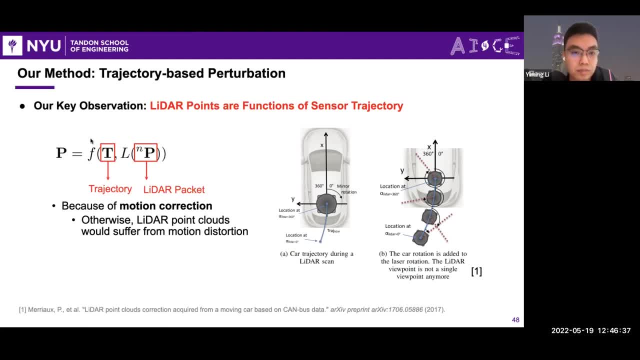 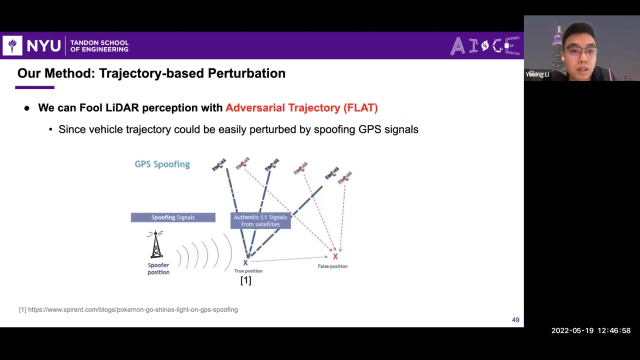 So, after get such kind of representation, our intuition that can we, instead of manipulating each points coordinates to achieve adversarial attack, can we manipulate the trajectory which is physically reliable to achieve the adversarial attack of the 3D perception, Because the sensor vehicle trajectories 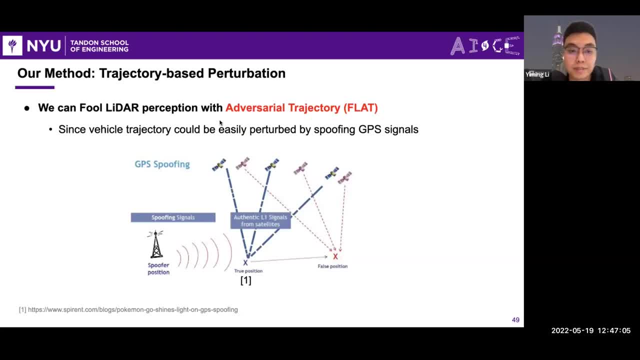 could be easily perturbed by spoofing GPS signals And so that we can full LiDAR perception. where adversarial trajectory perturbation, we can try to intentionally optimize some imperceptible noise onto the trajectories And we try to let the 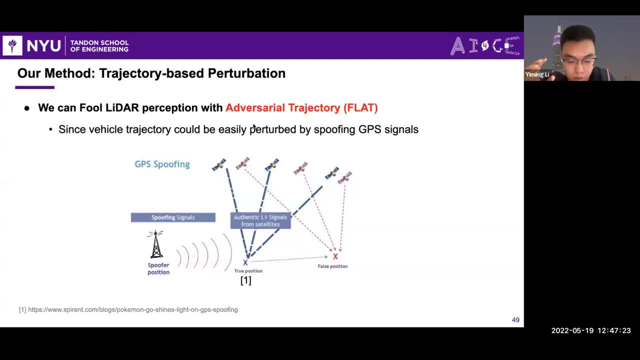 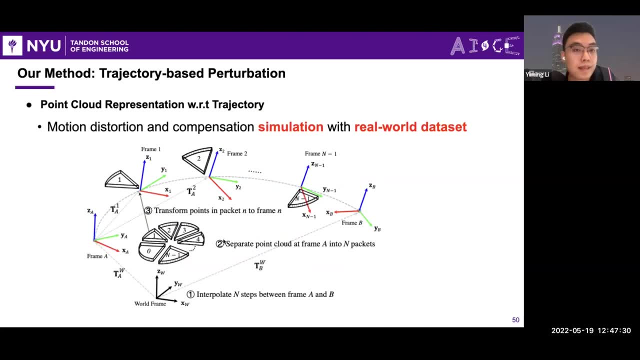 to change the point cloud so that deep learning model will be fooled by such kind of imperceptible trajectory perturbation. So to achieve such kind of method we need to, we first need such kind of data set. But, however, in the current perceptive data sets like PT, 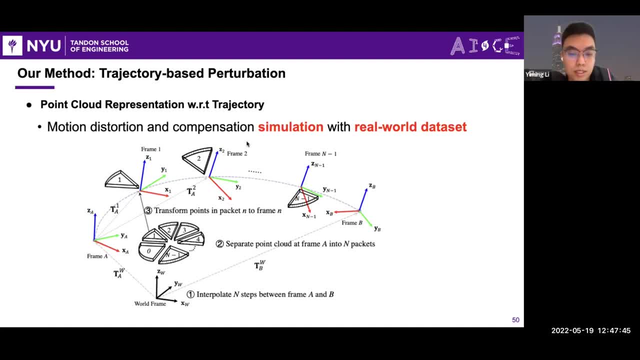 or new things. they all use the distortion-free point cloud, which means that they just have finished the motion distortion correction using the corresponding GPS information And however, we can try to simulate such kind of motion distortion and compensation right, Because we already know that. 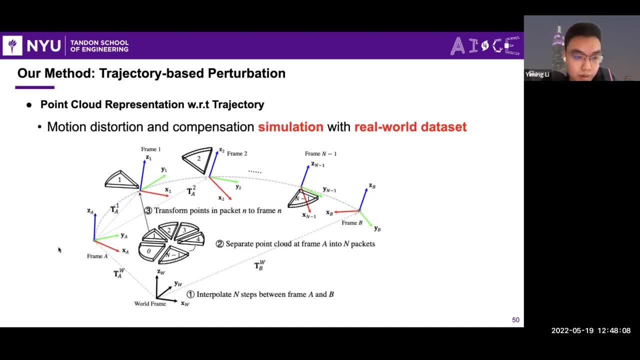 for example, we already know that frame A has its own full view degree of full view of point cloud And we also know its next frame is frame B. right, We know the corresponding pose, the corresponding six degree of freedom pose of the frame A and the frame B. 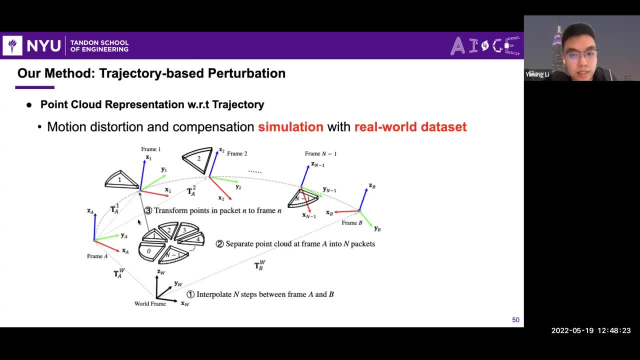 And we can try to consider the frame. the frame A's point cloud is captured at different locations. different trajectory points onto the trajectory which is from A to, which is from frame A to frame B, right, So that we can we assume that the vehicle is moving smoothly, right? 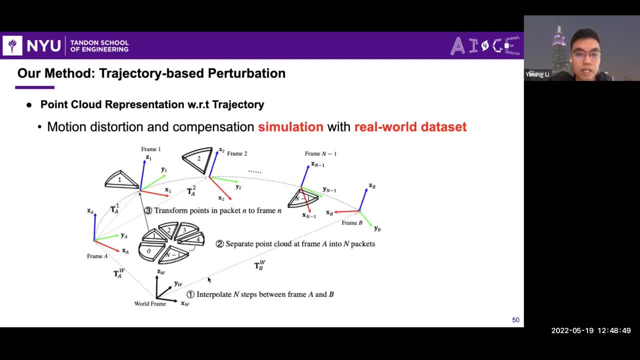 And then we interpolate N steps between frame A and frame B so that we can get- we can get N more poses right, And then we can. we can divide the point cloud at frame A into N LiDAR packets. Each LiDAR packet denotes a sector. 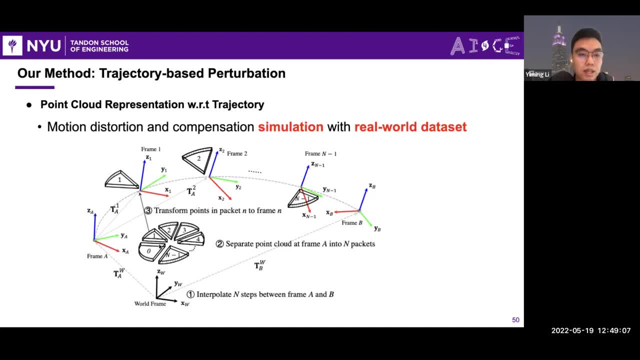 And it means that here the sector zero is captured at the frame A And sector one is captured at frame one And sector two is captured at frame two, And we also know the corresponding pose of different sectors, of different sectors, And these poses are simulated by our interpolation. 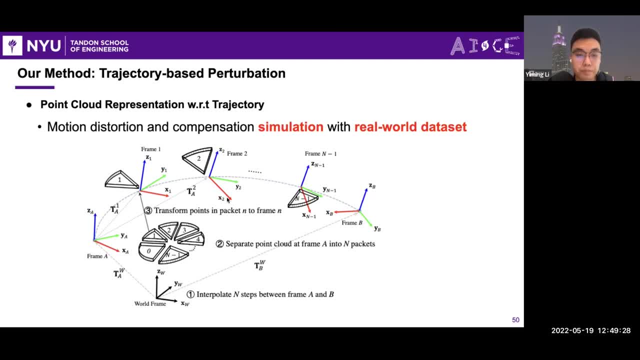 And so by such kind of simulation we can simulate such kind of motion distortion data set. You can see that here P denotes the point cloud at frame A, and it is aggregated from the different LiDAR packets, P and N, And P and N denotes 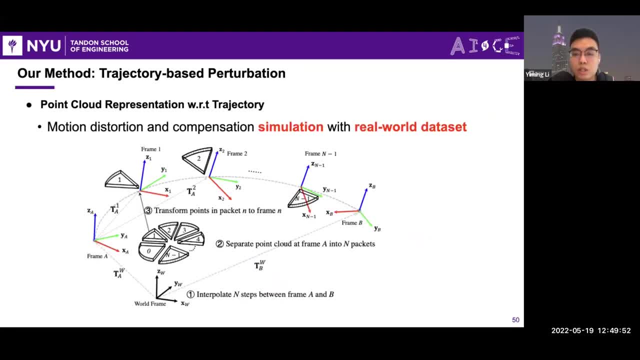 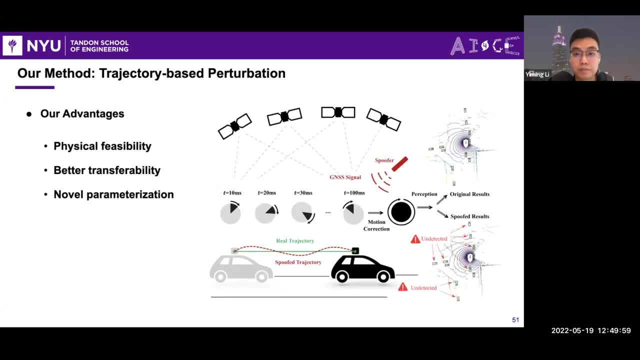 LiDAR packet captured at different trajectory points And we also know the trajectory T because we simulate such kind of trajectory by the interpolation. And compared to the coordinate-based adversarial attack, our method has several advantages. First one is physical feasibility. 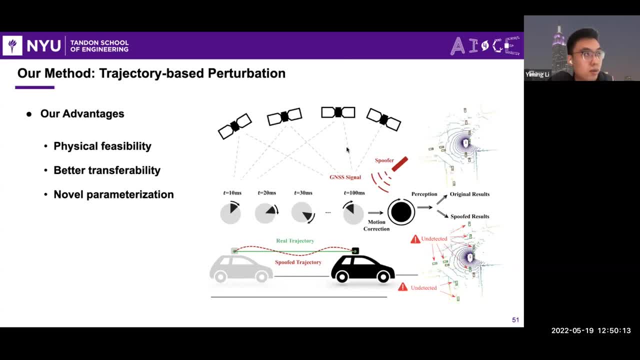 because the GPS spoofing is a well-studied error, Although we are not expert in that error, but we have do some literature survey and we found that that the GPS spoofing can be easily achieved. And second one is we have better transferability. 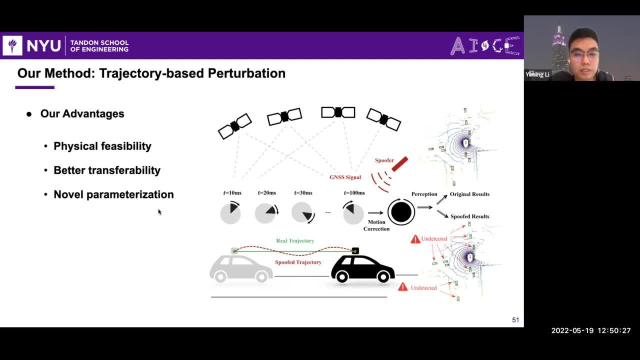 because our adversarial perturbation can even be transferred across frames. And for the coordinate-based adversarial attack, because the numbers of points is changing across frames so it is hard to transfer the coordinate perturbation across frames. But since our trajectory-based perturbation, 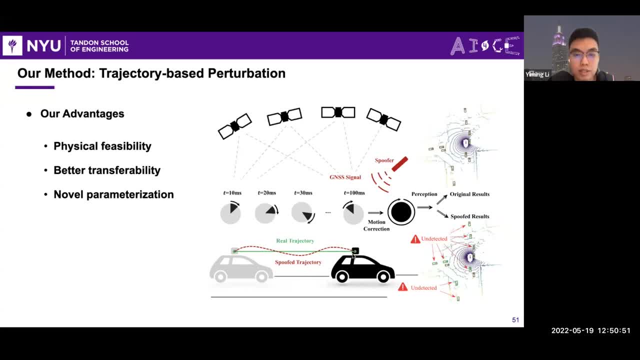 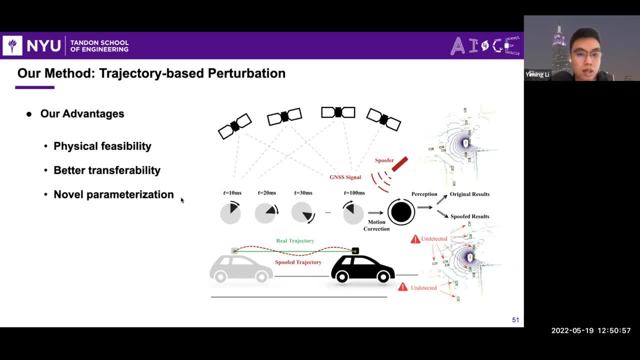 so that it can be transferred across frames. And also the most important one is that we have better attack performance due to the novel parameterization, For example for the coordinate-based attack. it's just try to attack single individual points, right, So we can only manipulate its X, Y, Z coordinates. 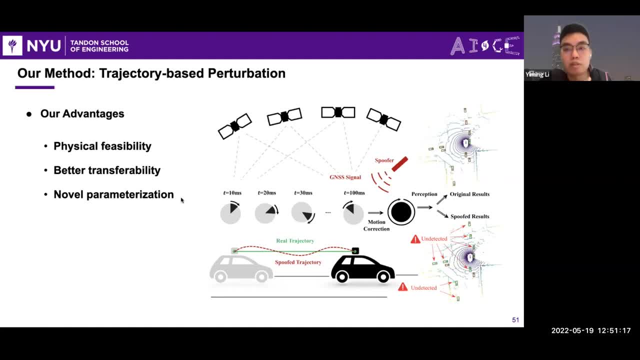 But for each sector, since we have implemented such kind of grouping and we can consider each sector, each LIDAR packet as a rigid body, right So that we can attack its orientation parameters, And so, in addition to the translational parameters, 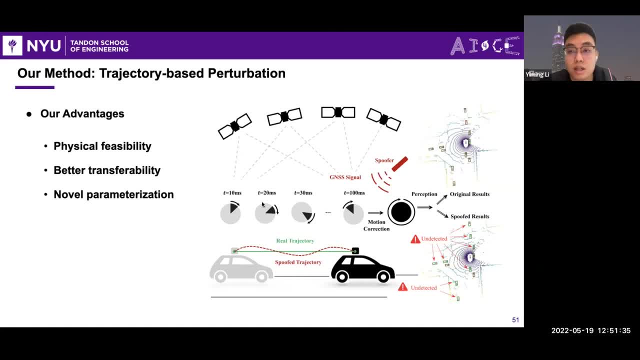 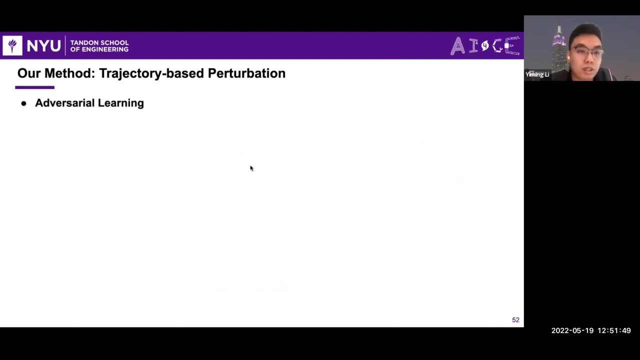 now we have a novel orientation of parameters So we can have a better attack performance because we can have better attack performance in our gradient-based adversarial attack framework. And now let me introduce our adversarial learning objective. And given a perception loss, which means here? it means that L denotes the detection loss. 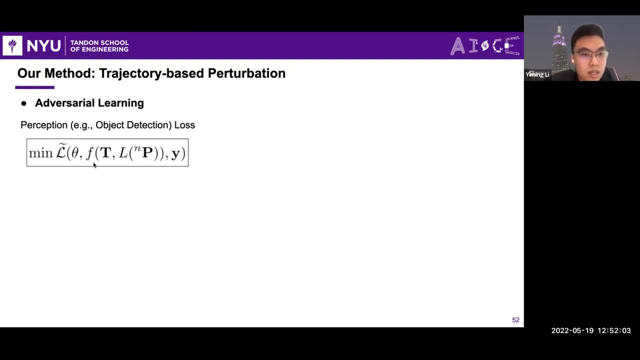 and the F is our deep learning model And it takes the point cloud as the input right, And our point cloud here is now a differentiable function of the trajectory, trajectory key And here Y denotes the ground truth labels, Which means that the ground truth bounding boxes. 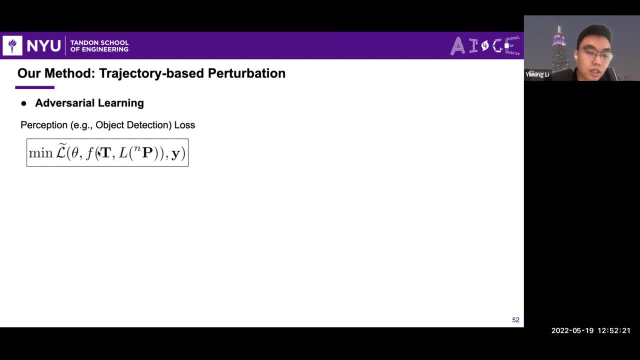 at each frame. And now we try to maximize the perception loss- right, Because the adversarial attackers are trying to fool the detector. So it is trying to maximize the perception loss, which is also means meaning that minimize the negative perception loss. 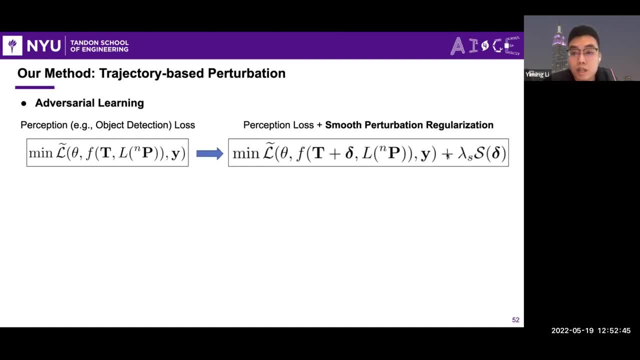 And in order to make our perturbation imperceptible, we have to use a method, And in order to make our perturbation imperceptible, And in order to make our perturbation imperceptible, we implement also regularizations on our trajectory. 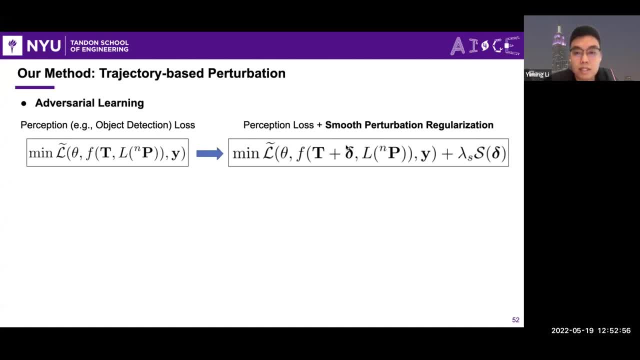 And here this data means the adversarial perturbations, And we will try to optimize that kind of perturbations And we also add a smooth perturbation regularization to try to make it very smooth, very imperceptible. And then we use the project. 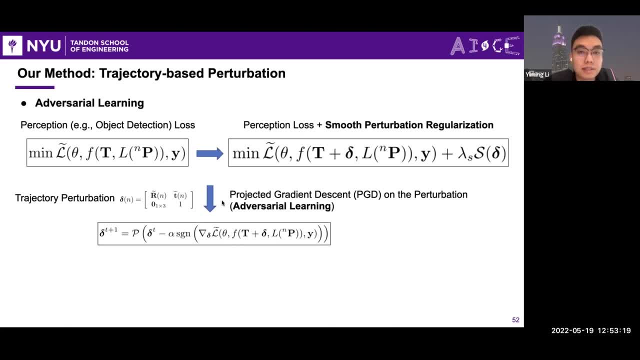 we use the descent on the perturbation And after our optimization we can get a very. after several iterations we can get a very imperceptible trajectory perturbation. And in order to make our perturbation highly smooth we also implement a polynomial interpolation. 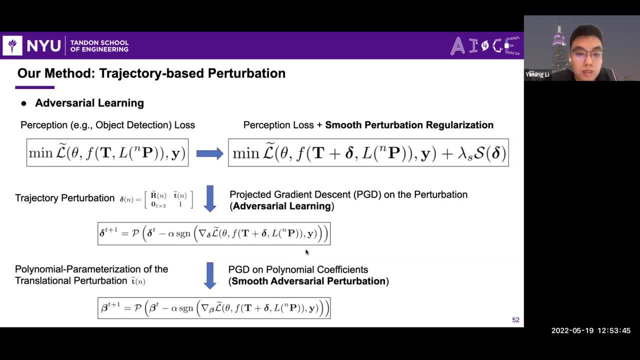 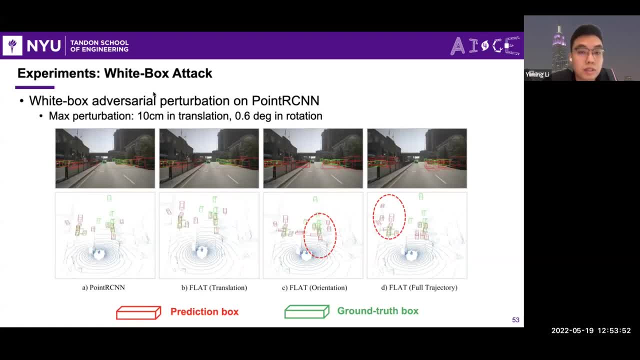 a polynomial parameterizations And I will show you the the performance later. And let me show you some experimental results. And here is our adversarial attack results in the white box attack. White box attack means that the deep learning models, the adversarial, knows the parameters of the white box. 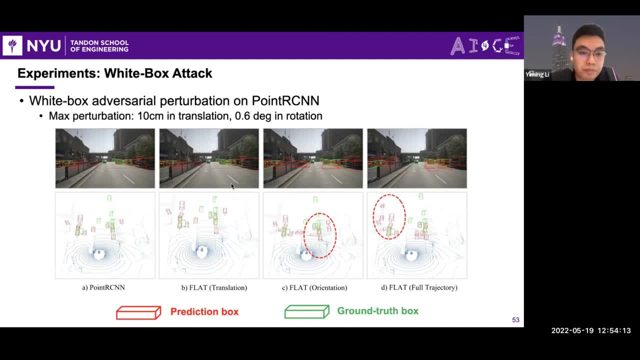 or the corresponding attack to deep learning models. And you can see that we we have, we have the our methods, which only attacks the translational parameters and orientation parameters, And also we have a full trajectory which means that we attack both translational 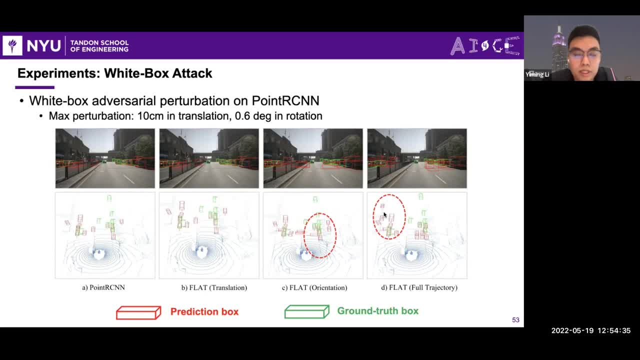 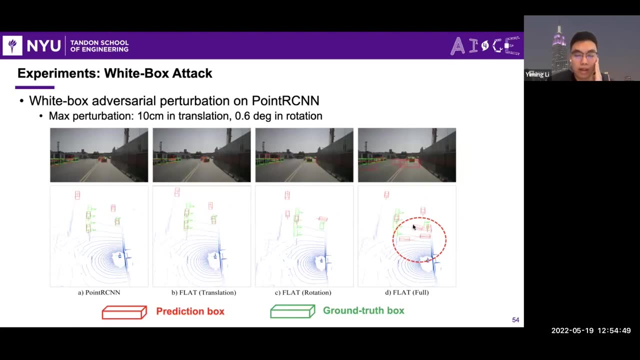 and orientation parameters. You can see that with more parameters attacked, there will be more false positives. You can see that here, red boxes denotes the predictions and the green box denotes the ground truth. And here is more results. And we have, we have. 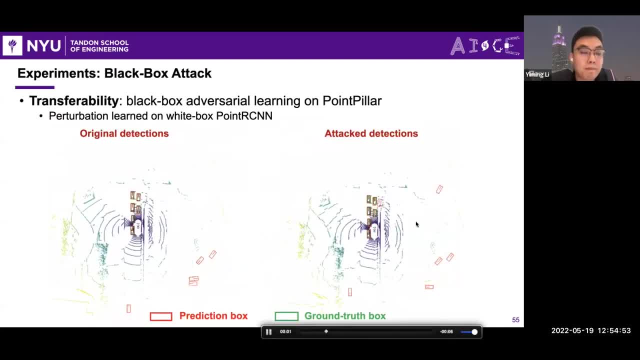 we can see the similar findings And we also conduct the transferability test, which means that we use the adversarial perturbation learned in the white box model And we transfer that kind of perturbation onto a black box model, which means that we do not know the parameters. 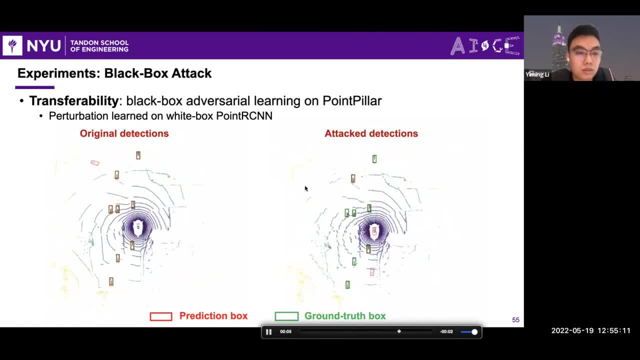 of the corresponding different models, And we just utilize such the perturbation learned by others. and we just utilize such the perturbation learned by others and we just utilize such the perturbation learned by others onto the black box model. You can see that here the 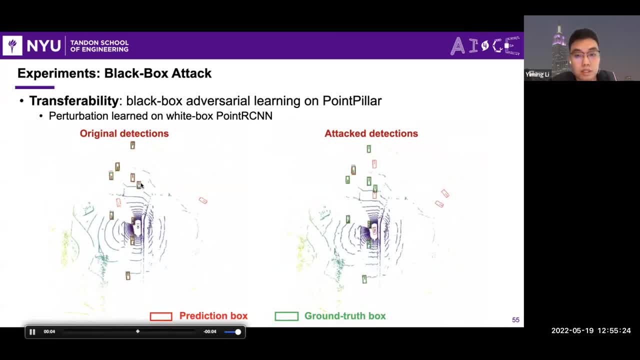 also, the predictions is denoted by the red boxes and the ground truth is denoted by the green boxes. Here the left video denotes the original detections and the right video denotes the detections after the attack. You can see that there are many boxes. many red boxes are lost. 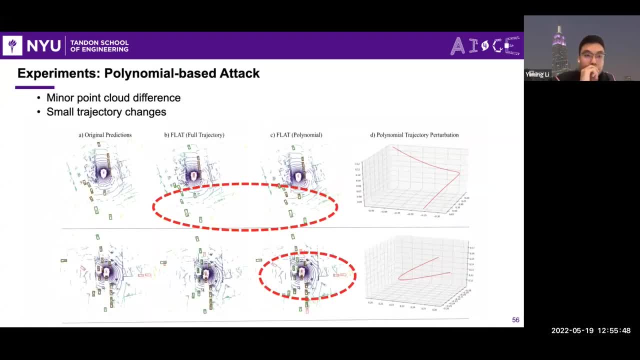 You can see that there are many red boxes are lost. And now let me show you our polynomial based attack. And our polynomial parameterization is that, instead of manipulate each trajectory point individually, we try to firstly conduct the polynomial interpolation to make it to make a trajectory perturbation. 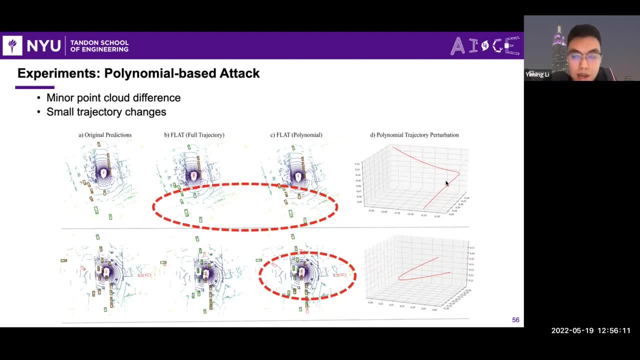 as three other polynomial functions, And then we try to manipulate the polynomial coefficients. And then we try to manipulate the polynomial coefficients to make it to make a trajectory perturbation as three other polynomial functions, And so so that we can achieve such kind of very smooth 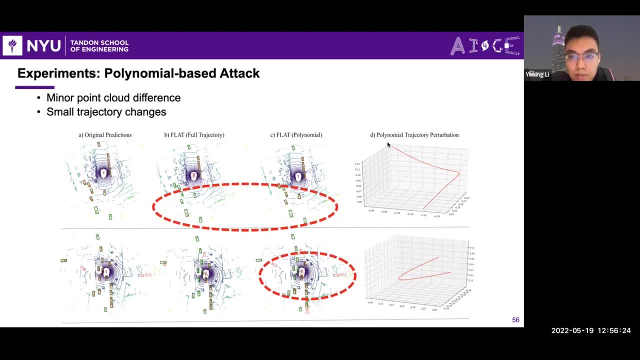 trajectory perturbation. right Here is the polynomial trajectory perturbation visualizing the 3D Euclidean space, And so it's kind of trajectory smoothness can also be reflected in the point. cloud space can also be reflected in the point cloud space. 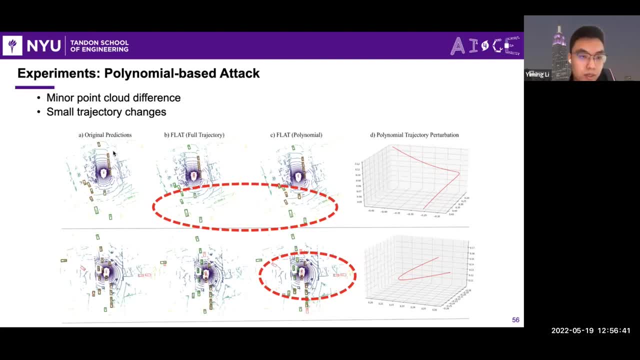 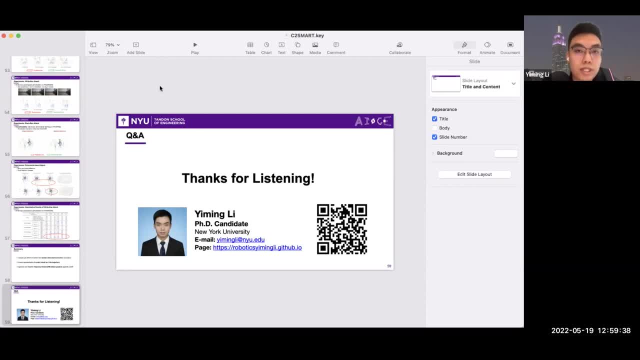 And after the point cloud you can see that the left figure is the original point cloud. Thank you, Thank you. Thank you, Dr. Okay to everything, communication right, And so everything can also involve both vehicles- roadside unit- and pedestrian trucks. 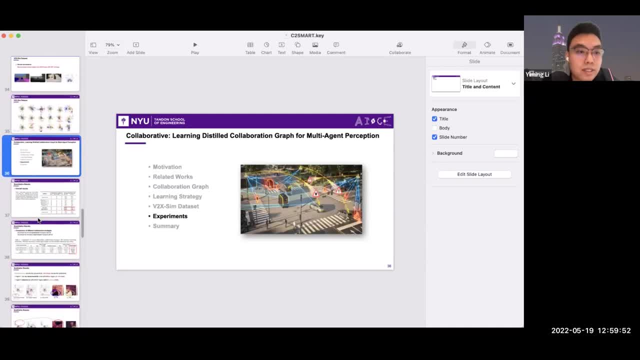 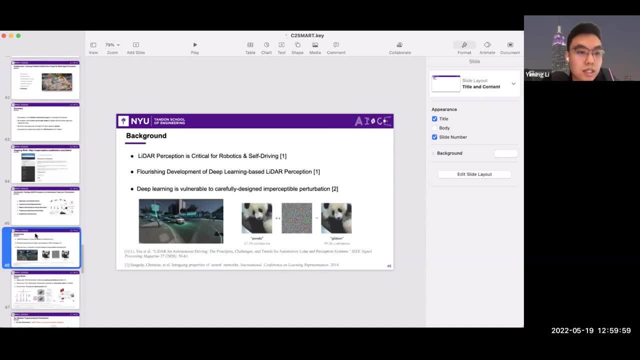 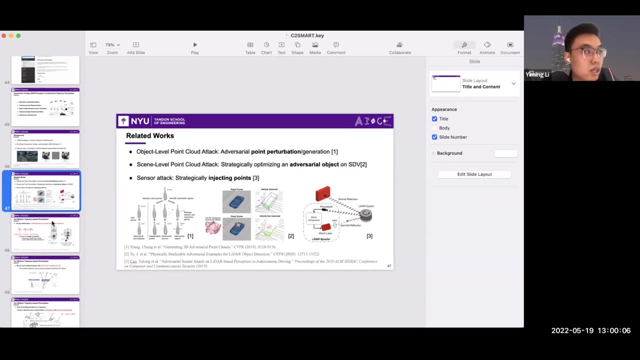 And, however, for our simulation we can only simulate the vehicles And I believe in the future, if we can simulate more elements such as pedestrians in our scene, we can actually try to think about that direction. Okay, and I guess, final question. 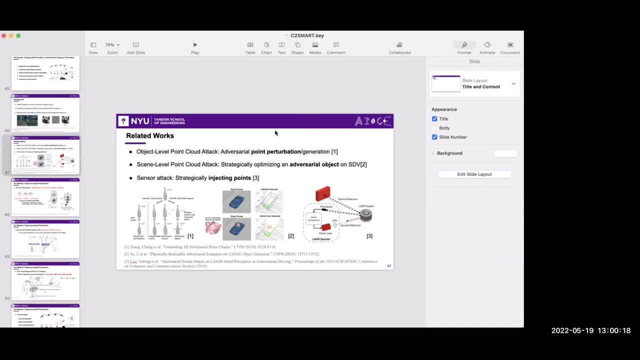 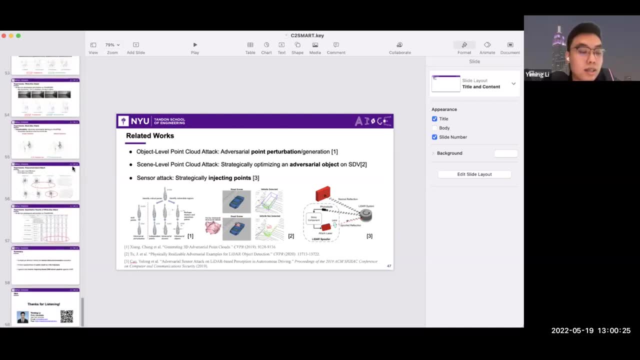 unless another one or two comes in in time. So can you tell us again a little bit more about what you're working on right now and why you're excited about it? Okay, currently we are still for the first part of collaborative perception.